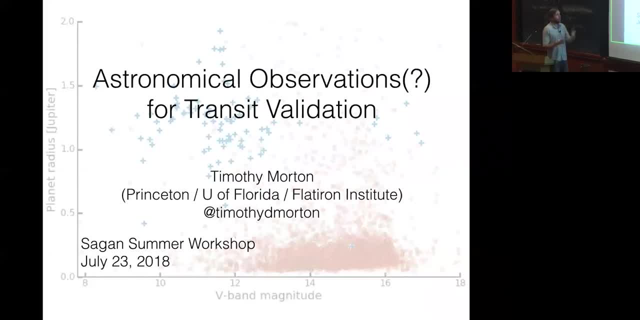 Good, Okay, Great, Yeah. so I'll be talking about, like everyone else I'll be, you know, focusing on transits today- My multiple affiliations here. I've been at Princeton. I'm starting as a faculty at University of Florida this coming year. 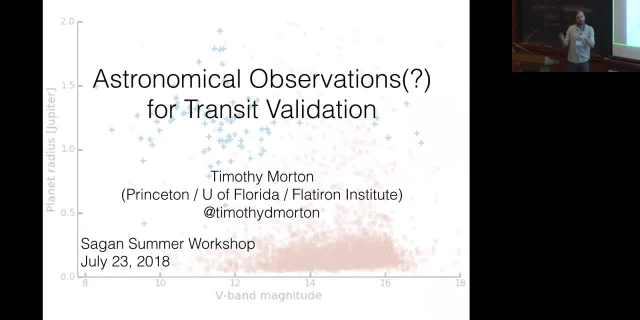 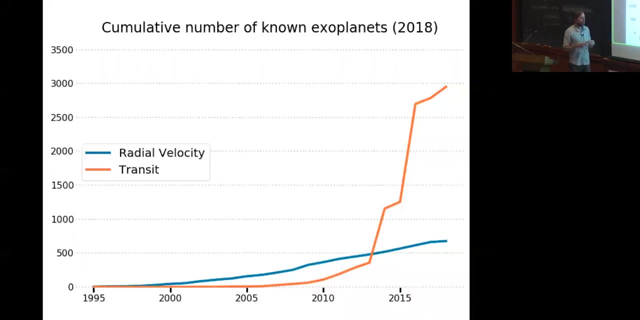 So that's. but this year I'm also visiting the Flatiron Institute in New York, So that's just a multiple affiliations situation here. So what I'm going to cover in this talk essentially is how the field of exoplanets, or specifically how the field of transiting exoplanets, came to really dominate the field of exoplanets just over the last few years. 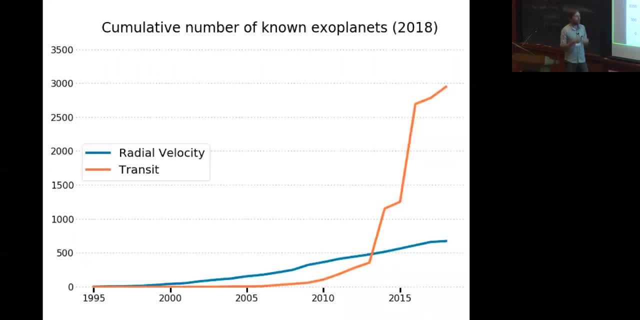 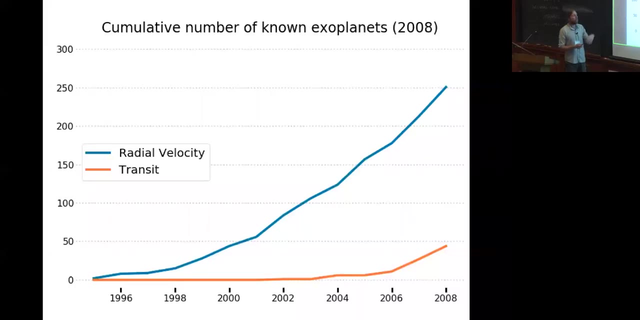 And sort of you know what happened such that you know it sort of started to take over and you know a little bit of the background there. Sort of zooming in on earlier a few times, when I was starting as a graduate student here, this is what the field of exoplanets looked like. 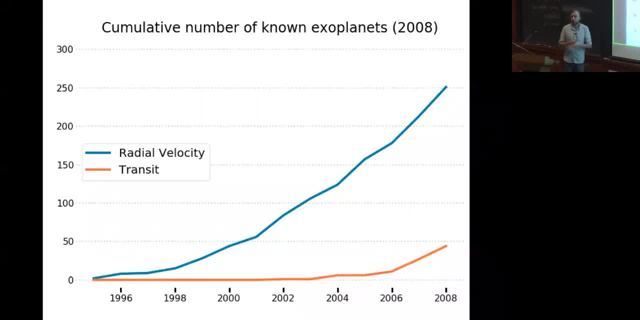 So you know very different situation. All of you guys have been raised in the Kepler era. I was sort of at the very beginning of Kepler. you know when I started. But you know really. you know 10 years ago transits was sort of like a niche market of exoplanets at large and radial velocities was really the dominant force in town. 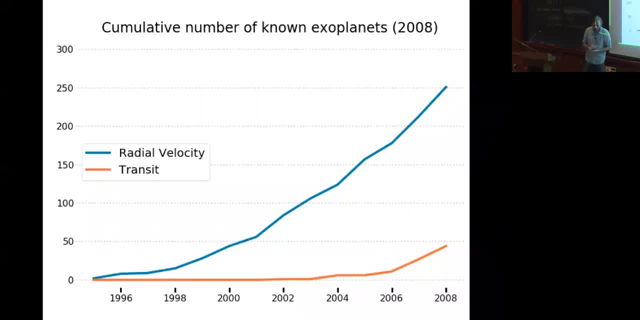 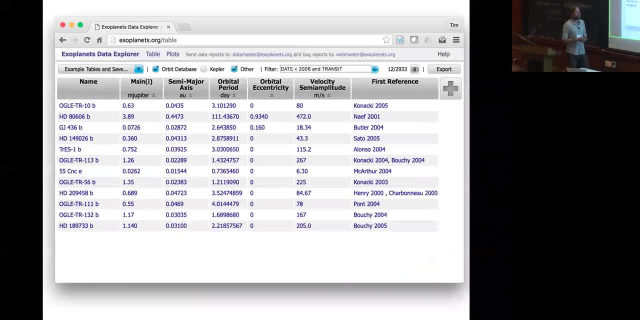 So what I'm going to start by doing is, you know, do a little bit of an exoplanet history lesson For those of you who haven't, you know, lived through this. at least you know academically. 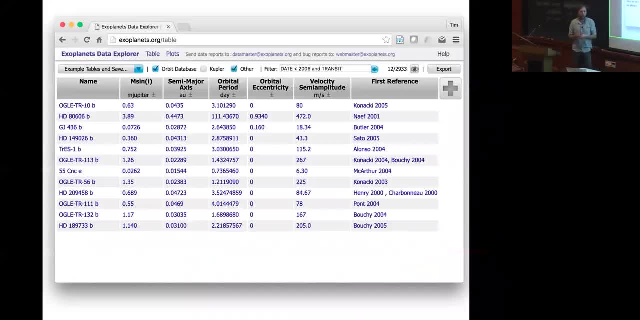 These are the planets that the transiting planets that were discovered prior to 2006.. Okay, There's a list of like 12.. Three of them were discovered. the planets themselves were discovered prior to 2006,, but they weren't yet known to us. 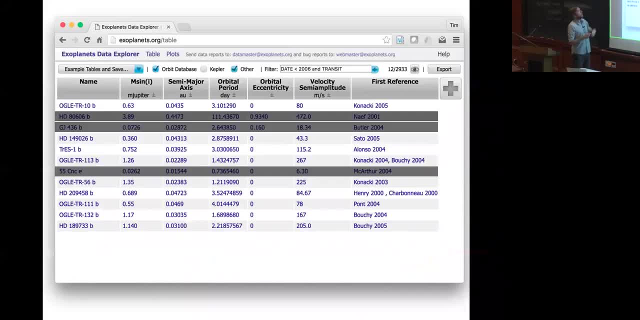 They were discovered prior to transit, So I've graded those out and the nine planets left. there are the only transiting planets that were known in 2006.. So the first one I'm going to talk about here is Ogilv, TR 56b. 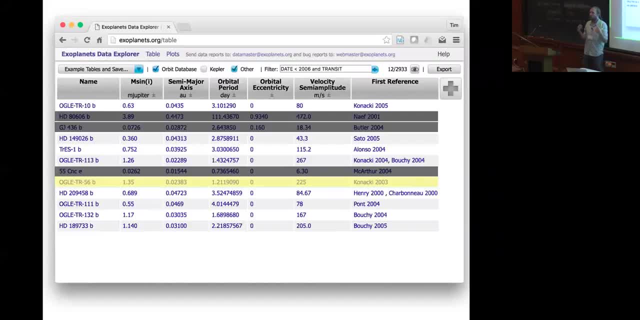 The distinction of this planet is: this is the very first planet that was detected by its transit. So HD 209458b was the first detected transiting planet, But it was first detected with radial velocities And it was subsequently observed to transit. 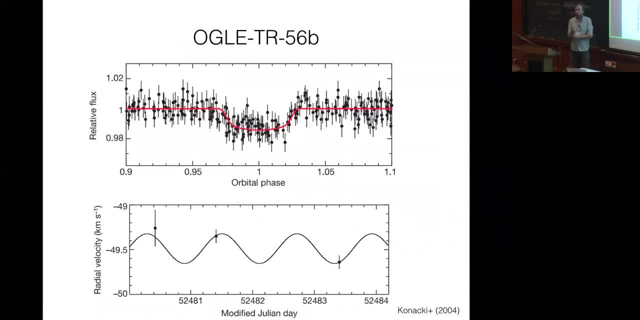 So Ogilv TR 56b. This is the discovery data. All of you who work with radial velocity data these days, this is the discovery, like the discovery radial velocity curve, The radial velocity confirmation curve for the first transiting exoplanet discovery. 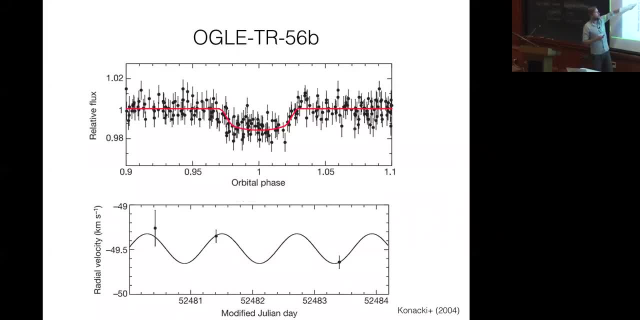 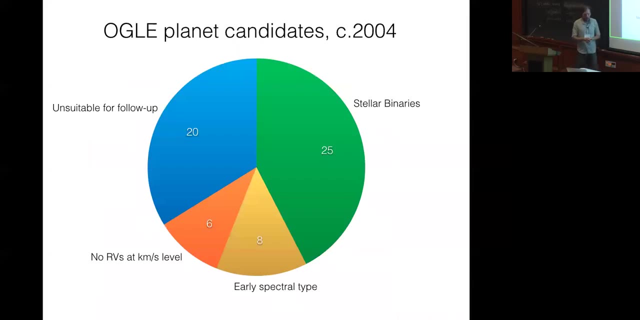 We see three points And you notice that these units are in kilometers per second. So you know, this is a very different ballgame from what we're doing these days. But you see, the top is the phase-fold optometry And this is the confirmation radial velocity curve. 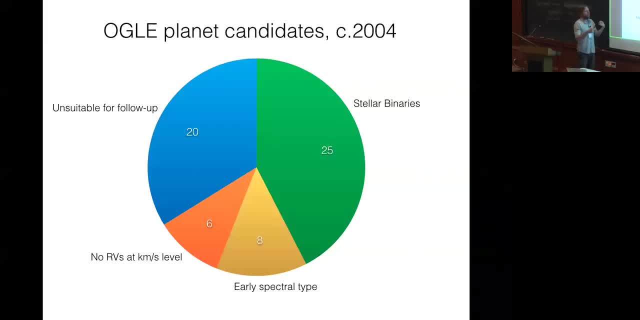 This particular planet came from this set of candidates. So Rafael talked earlier that you know many transient surveys will detect lots of things that look like they might be planets but only a small amount end up being confirmed planets at the end. This is sort of what that pie chart looks like for the Ogilv detection. 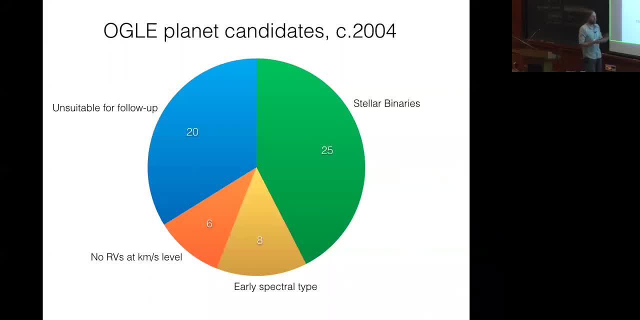 So you know, they found over 50 candidates. About 25 of them turned out to be stellar binaries of some sort. Eight of them were detected to be rapidly rotating stars, which means you can't do precise, or even moderately precise, radial velocities on them because they're rotating so rapidly. 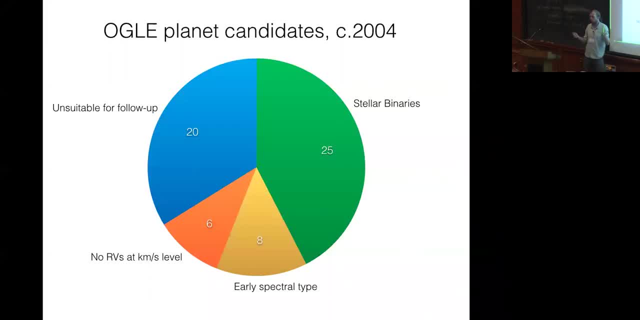 And then there were you know 20 that were, you know, unsuitable for follow-up for various reasons: Maybe the stars were too faint, Maybe it's too crowded. The Ogilv survey is a microlensing survey, So it was designed to look for microlensing events. 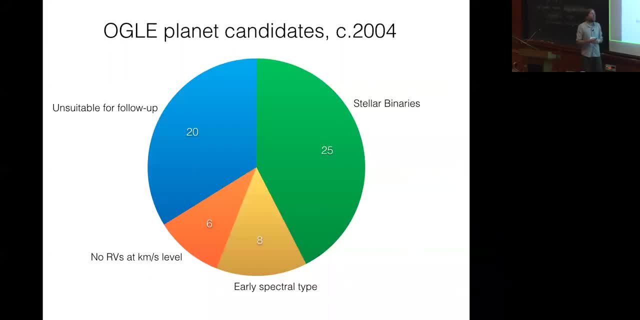 So it wasn't specifically designed to find transiting planets. But you take similar kinds of data so you can find planets in that. But because it's microlensing field, it's a very crowded field. So you know, maybe some of these were too crowded to do follow-up. 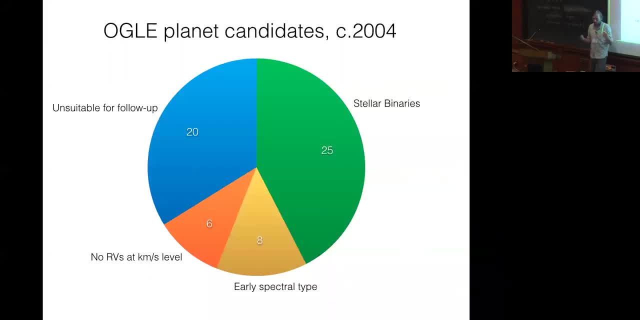 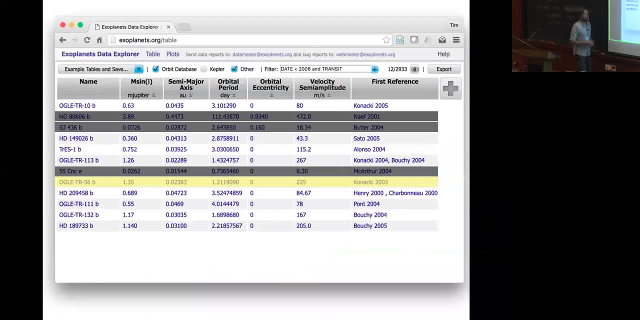 But six out of these turned out to not have significant radial velocity variations at the kilometer per second level, which means they were not existing binary stars and they could be planets, And so Ogilv TR-56 was one of those, And there are the other ones here. 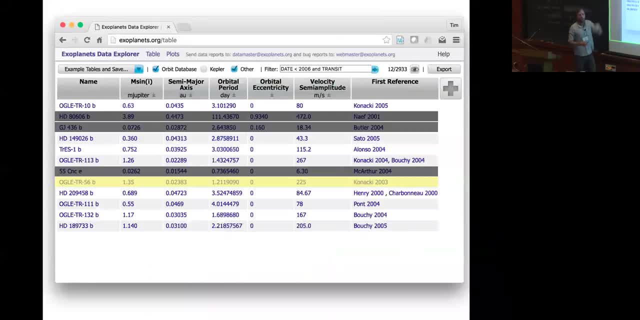 One, two, three, four. One, two, three, four, five were other Ogilv planets there, And we noticed there weren't six of them. The next system I want to talk about is Ogilv TR-33, which is not on this list. 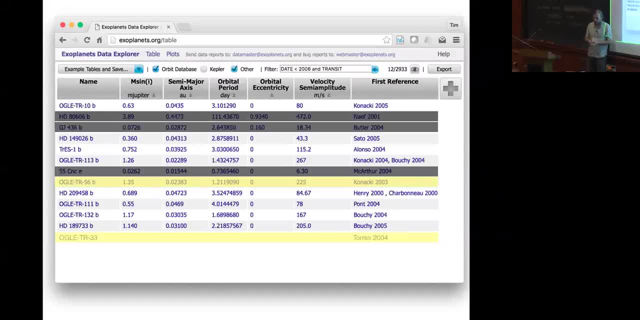 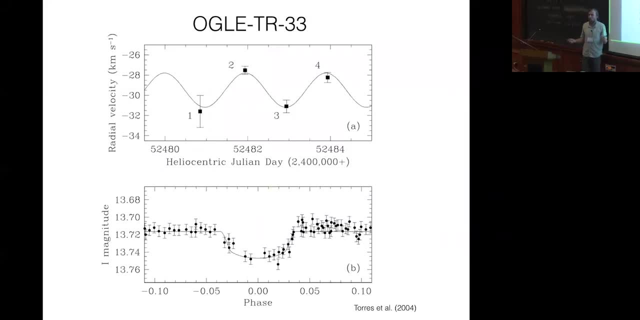 You won't find it on exoplanetsorg for reasons that will become apparent very soon. This is the discovery data for Ogilv TR-33.. It looks very similar to the first one we saw. We have a, you know, phase fold of photometry, a dip of a couple percent. 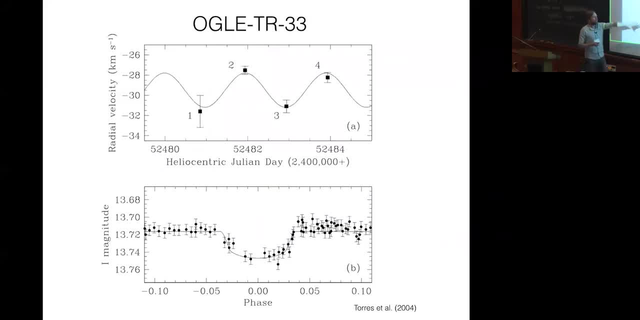 You know it looks like a Jupiter, A Jupiter-sized planet, And the radial velocities you know very indicating. you know a few Jupiter mass planets as well. But it turned out that you know, on further analysis of the shape of the spectral lines, it was determined that this is actually a hierarchical triple eclipsing binary system. 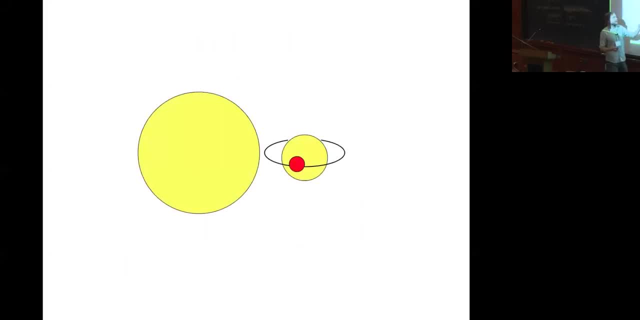 A particularly nasty one because the bright this is a G subgiant and a G dwarf. The G dwarf was being eclipsed by a smaller star, And the reason it's particularly nasty is because these two stars have the same color. So they even did, you know, multiband photometry, you know like looking at the transit depth in different filters, and it checked out. 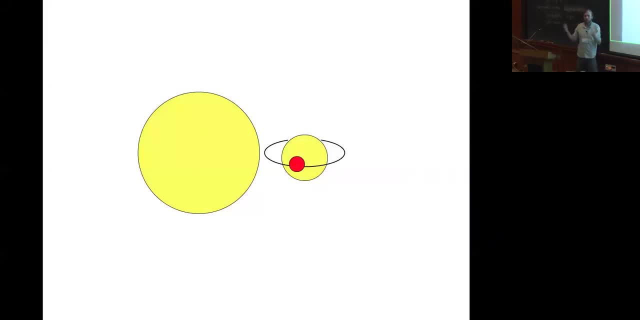 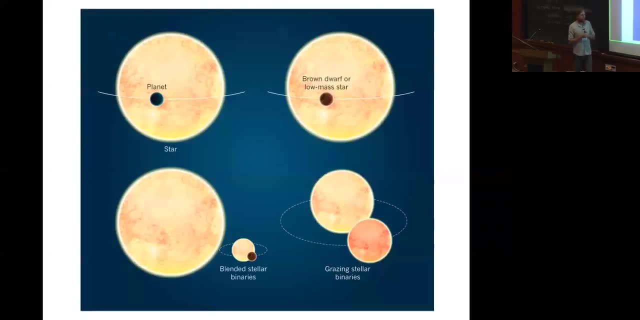 So this is. this became kind of the poster child of the scary astrophysical false positives that you can get from transit surveys. This is Ogilv TR-33.. And again Rafael showed a slide similar to this. This is kind of the family portrait of the common astrophysical false positives you can get in transit surveys. 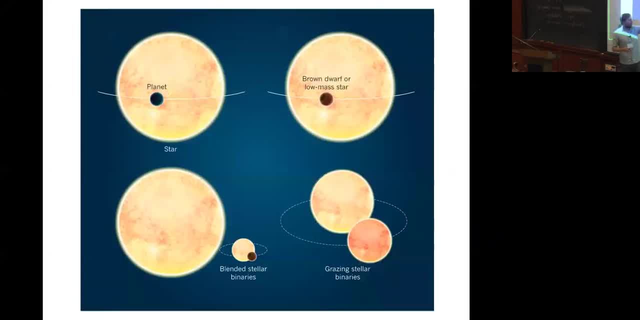 So this is like the Ogilv TR-33 system, where you have a blended eclipsing binary where the depth of the signal is diluted by this brighter third star. This eclipsing binary can be either physically associated, as it was in the Ogilv TR-33 system, in a physical triple system. 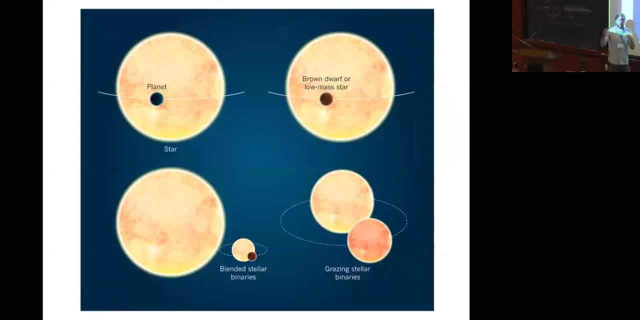 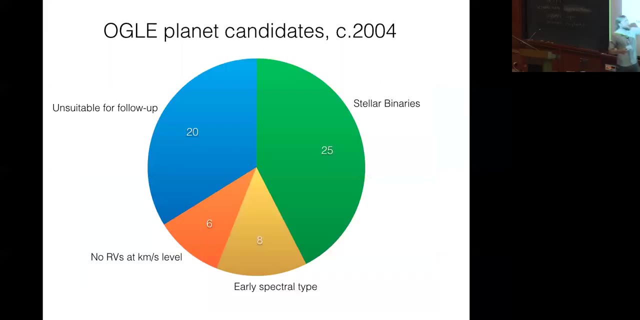 Or this might be just a chance alignment of another star in the foreground or background, You know, unrelated to the primary target star, And then you can have these grazing, eclipsing binaries, or an eclipse of the low mass star or brown dwarf. So again, so all of the you know, the things that turned out to be stellar binaries. 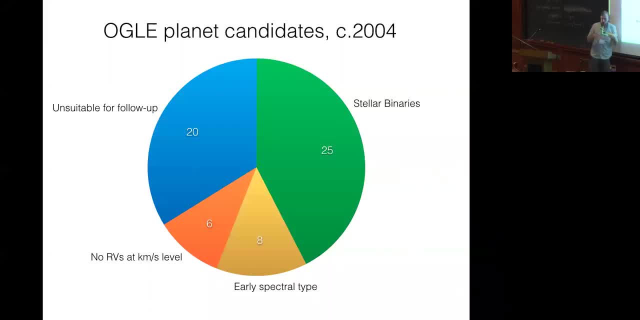 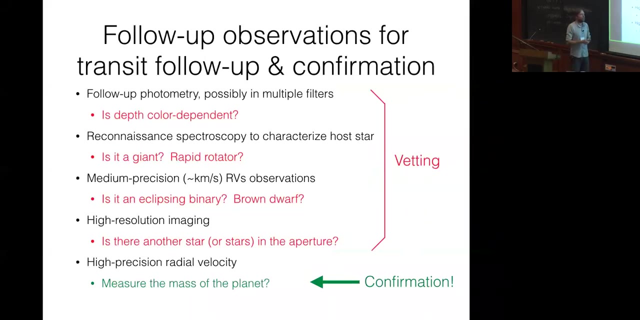 And probably some of these two were things that you know fell into those false positive scenarios. And the way, the procedure that the astronomers went through to kind of whittle all this down is, you know, this procedure of you get a set of candidates from your discovery photometry, from your survey. 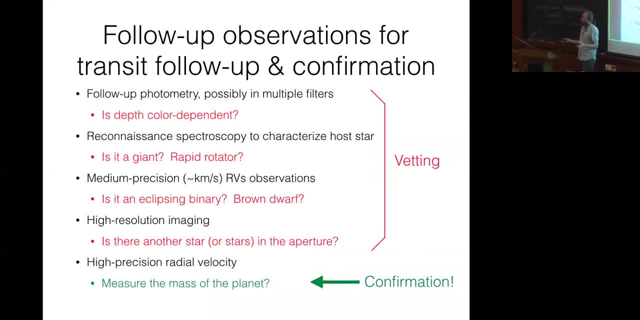 And then you do lots of different follow up observations to try to rule out various false positive scenarios. So you know you can. you know these vetting steps aren't in any particular order, But you know you can do follow up photometry with perhaps higher signal to noise than your discovery data. 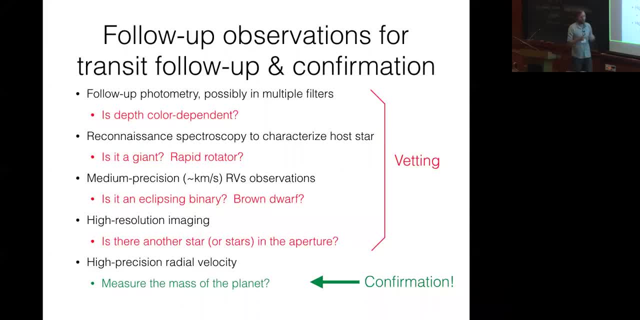 You try to measure the shape of the transit more precisely Or measure it in different band passes to look to see if the depth is color dependent. Do spectroscopy to characterize the host star, to see if it's a giant or rapid rotator. You can do medium precision radio velocities to see if you see, you know, a large rate of velocity variations from an eclipsing binary star. 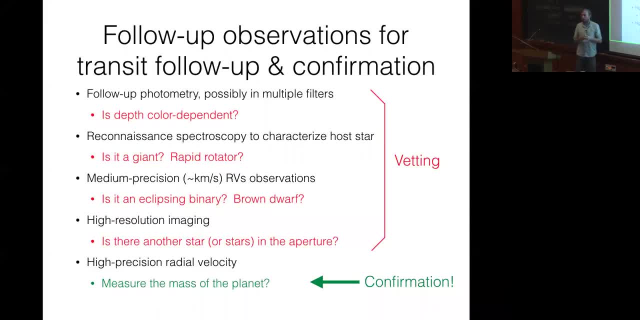 And you can also do high resolution imaging to see if there are any blended stars in the photometric aperture, To see if there could be. you know any false positives from that And so, like you know traditionally, you know the way this goes with these transit surveys is that you do all these vetting steps. 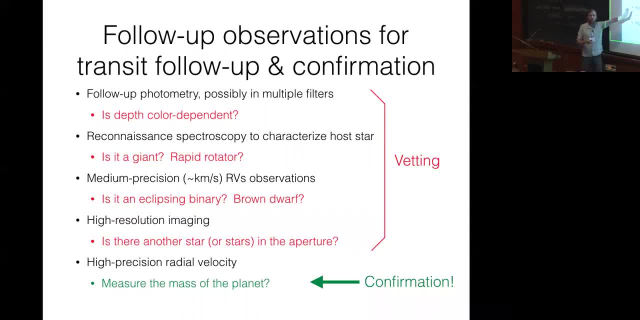 And you end up with a much smaller list than you start. It's that like wedge of sticks that we saw on OGLE, And then those are the candidates that you can afford to send to your big telescopes. You know, high precision for high precision radio velocity measurements. 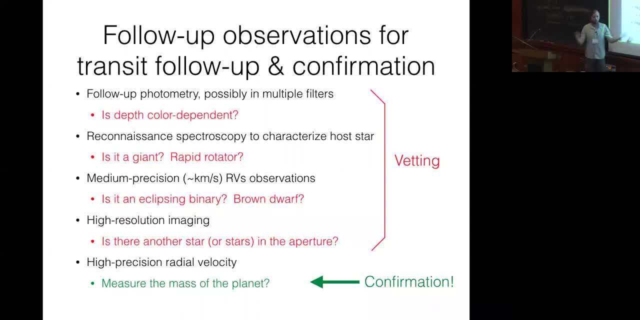 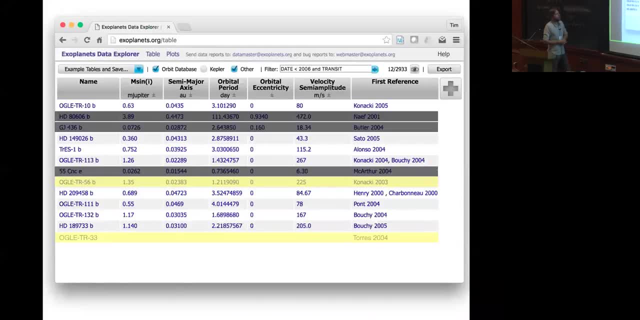 And you know, eventually, with a goal of measuring the mass of the planet, to confirm it as, yes, this is true, This is a bona fide planet. So the last sort of history planet I'll talk about here is TRACE-1b. 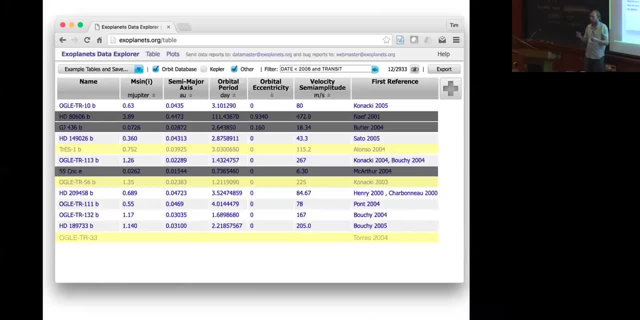 TRACE-1b was the first exoplanet that was discovered by a survey that was designed to find transient planets. So for the OGLE survey the transient planets were kind of a side benefit from, you know, the primary mission, which was microlensing. 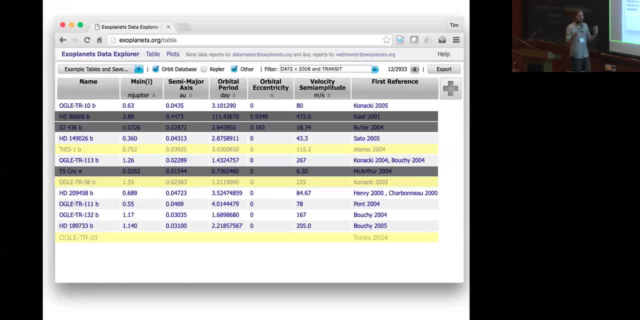 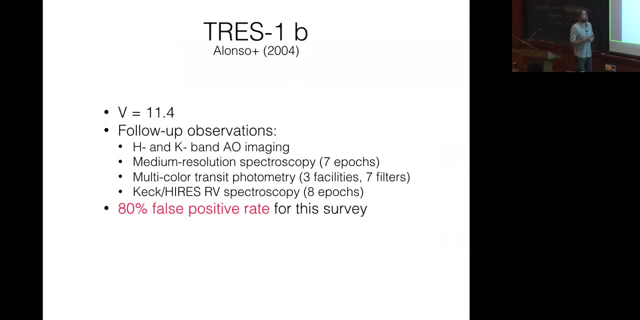 And the TRACE survey was designed specifically as a wide field, ground-based transient survey to find planets, And this is a precursor to the HATNet survey And this is what went into the discovery of TRACE-1b. So it's a, you know, relatively brightish star. 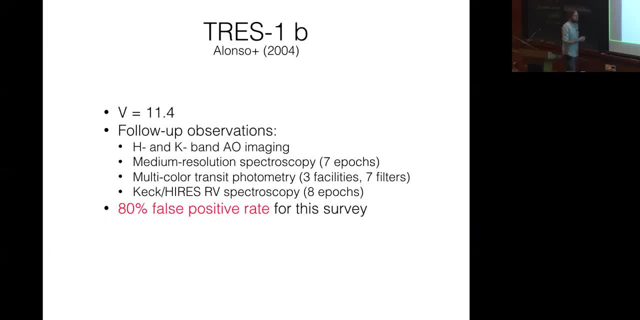 And you know, follow-up observations were, you know, multiple high resolution images, Medium resolution spectroscopy, Photometry in different bands to look for, you know, color-dependent transits And finally the confirmation spectroscopy to measure the mass of the planet. 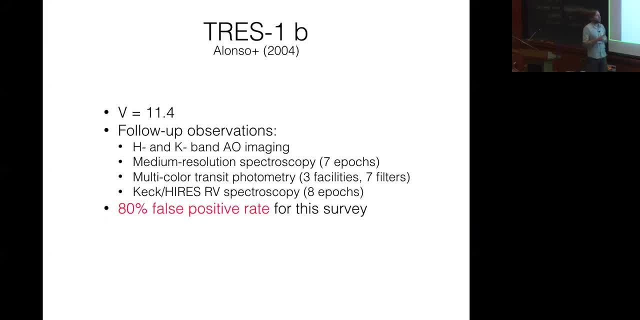 And for this particular survey, you know about 80% of the candidates that were sent to this follow-up procedure sent for follow-up observations. about 80% of them turned out to be false positives. So again, this is really a false positive dominated landscape that we're talking about. 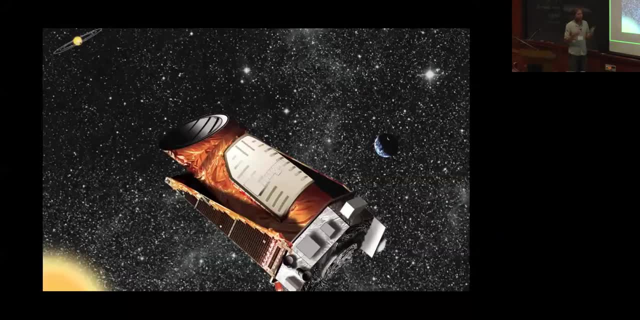 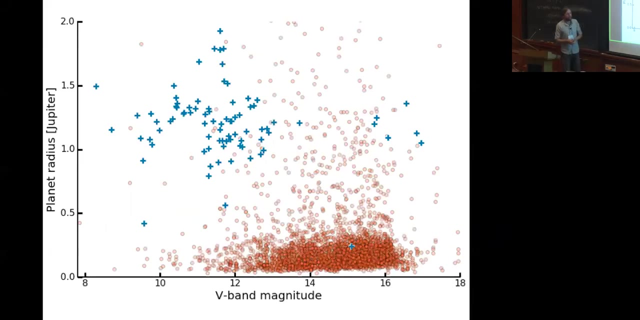 Back in these days, And now, of course, we're in the era of Kepler, And Kepler introduced new issues into the field of you know what do you do with exoplanet candidates? And those issues are summarized by this figure, which is showing the size of the planets on the y-axis and the brightness of the host stars on the x-axis. 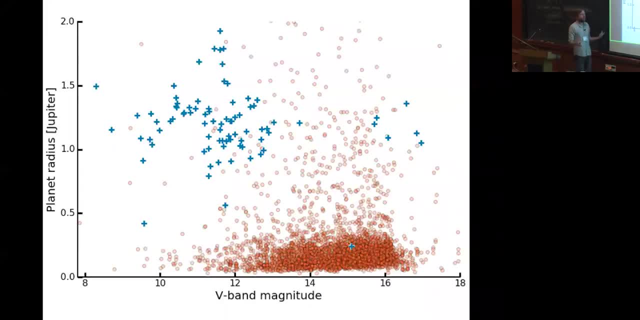 And you see, Okay, So right off the bat, there's three things that are, you know, that are totally new with Kepler. The first thing is that you notice that, you know, most of the stars are significantly fainter. 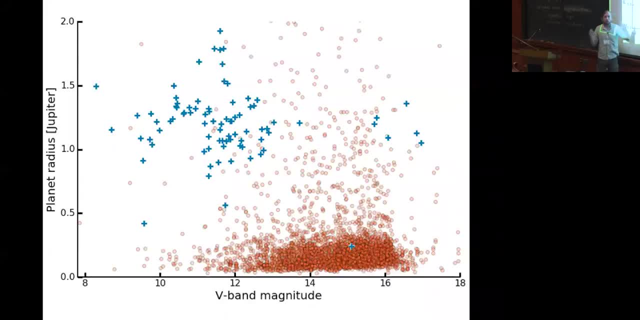 So I should explain what the points mean. The blue crosses are the ground-based transiting planet detections prior to Kepler, And the orange circles are the Kepler candidates. So you notice that Kepler candidates are, you know, almost all around significantly fainter stars. 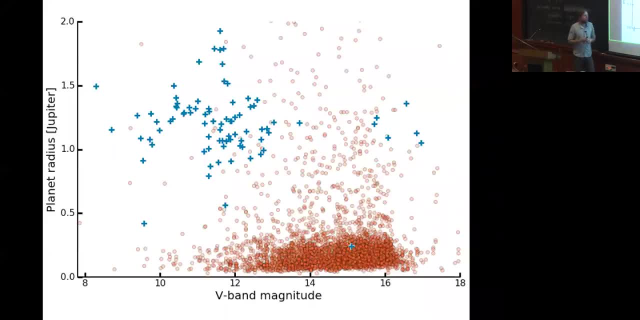 Than the ones that were found with the ground-based surveys, And also the vast majority of Kepler candidates are much smaller planets than the giant planets, primarily, that were found from the ground. So what that means is that you know, if the end goal of your train of follow-up observations is to measure the mass with radial velocities, you're out of luck, for you know 95% of these planets. Because you know, even with all the telescope time that you could ever wish for, you wouldn't be able to measure the masses for most of these. And then, of course, the final issue here is that there are thousands of Kepler candidates. 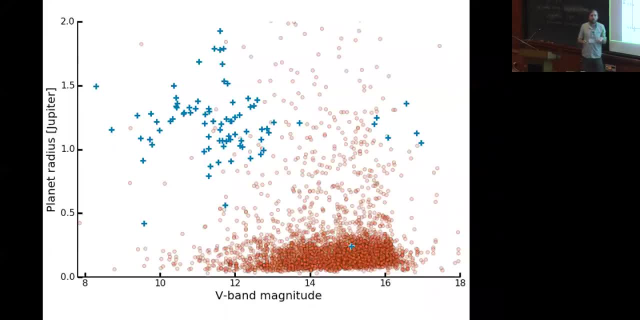 And there were about 100 planets, ground-based transiting planet detections from the ground prior to Kepler. So there's stars are faint, planets are small and there's thousands of them. So you need- you need something else to do. 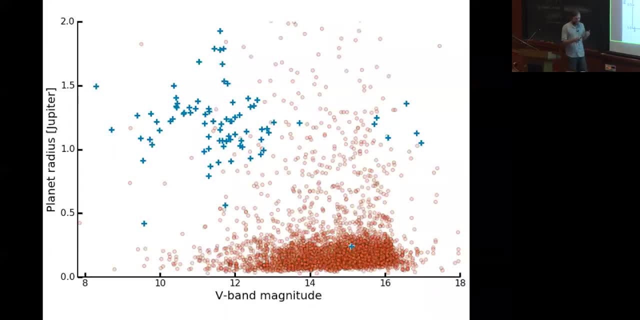 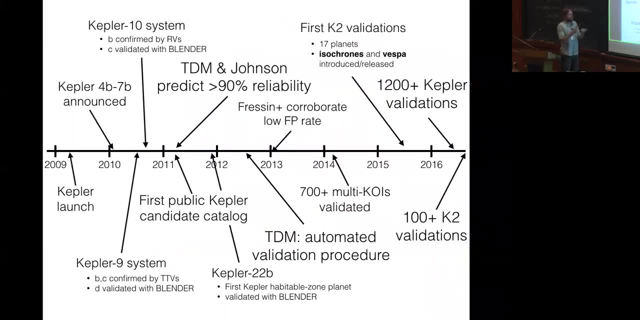 The. you know business as usual isn't going to work, And so what? I'm going to kind of go through the rest of this talk here, Okay, So what I'm going to go through here is this timeline here. I'll sort of step through it piece by piece. 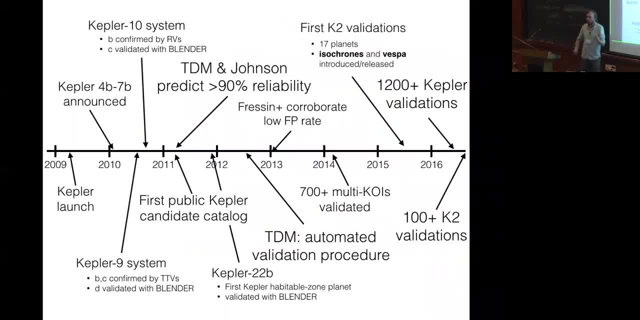 But this basically kind of shows the evolution of the kind of paradigm of how to deal with transiting planet candidates from Kepler launch to, you know, to present day. So at the beginning here, the very first discoveries that were announced by Kepler were very much in the traditional, in the traditional manner where you know these were relatively bright stars. 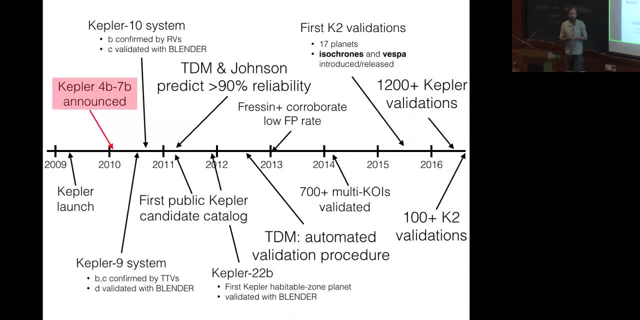 You know, Kepler found thousands of candidates, Some of them were around bright stars. So, these relatively bright stars, they were followed up with radial velocities. They got, you know, radial velocity masses, just like we're used to. And so those were the first four Kepler announcements that were made in the at the AAS meeting. you know, following the Kepler launch, you know, about a year afterwards. 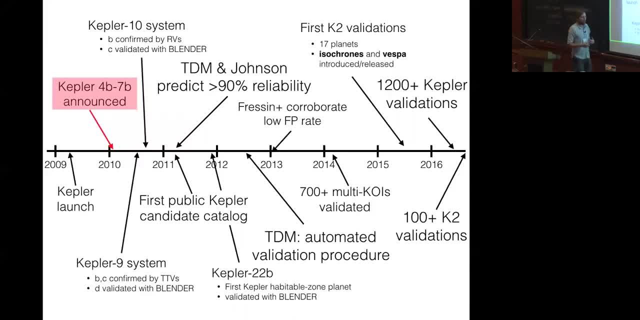 And sort of you know past that things started to get a little bit more. you know innovations started to become necessary To find more planets from Kepler, Just because the radial velocity follow-up was not going to turn out. you know very many more in any sort of reasonable amount of time. 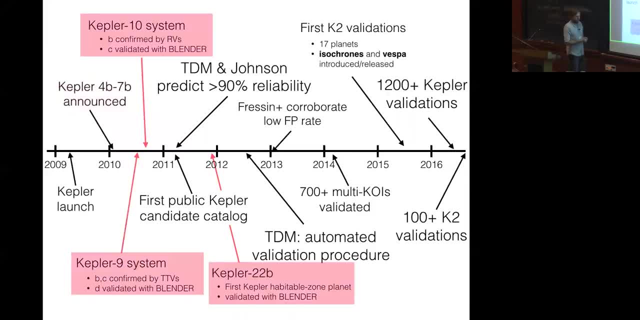 So you know, a lot of these early Kepler planets were found, as Dan was talking about earlier today, by transit timing variation. So you know the first of those was Kepler-9- here where two of the planets in Kepler-9 were confirmed with two TVs. 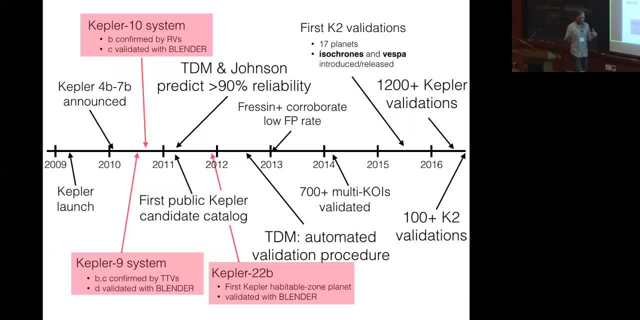 And then the third was with this other, this new technique which sort of broke the ground for this new way of thinking about transiting planet candidates. And what happened with Kepler-9D was it was probabilistically validated using a procedure called Blender. 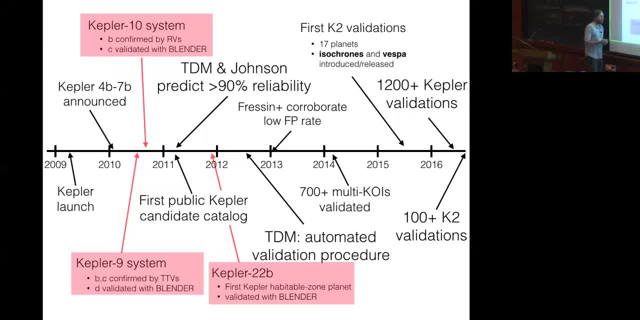 A Blender was sort of born out of the kind of analysis that went into figuring out that Ogilv CR33 was a false positive. So the same people who sort of dug into that and figured that out. You know, it's a little bit more complicated. 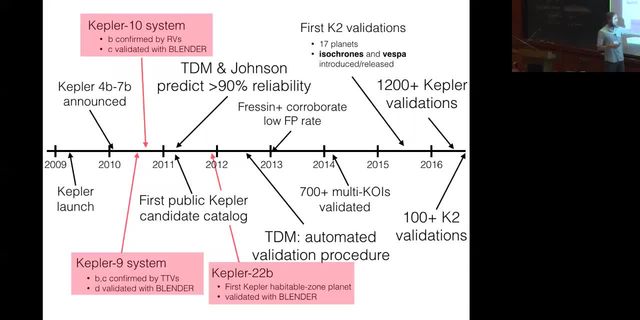 But it extended that methodology to be able to apply to Kepler candidates in this Blender tool, And so, after this one, a lot of the Kepler discoveries were announced were validated using Blender, And this terminology that I'm using and that several other people have used so far today is like confirmation versus validation. 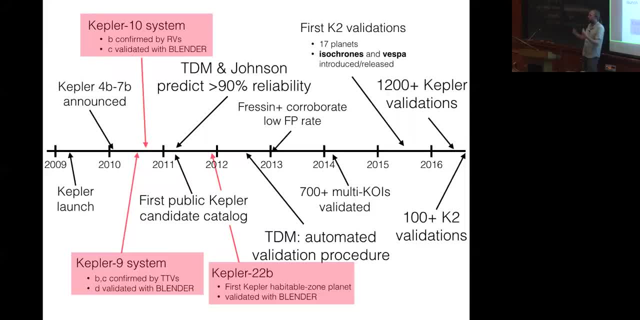 If that's confusing for anybody, it's okay. You know, It was like invented in these days here, You know, So it hasn't been around for very long. Usually, when we talk about confirmation, we're talking about sort of you know, dynamical proof that the candidate has a planet mass. 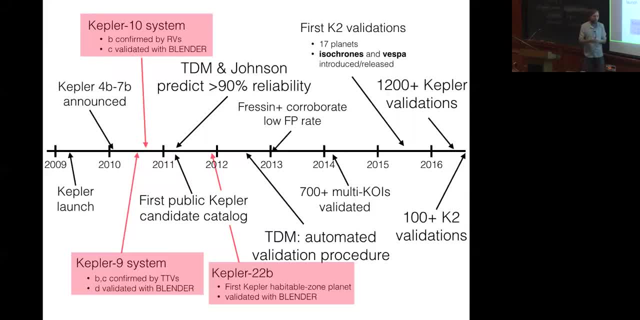 So, like you know, TTV measurements or radio velocity measurements- we consider those to be like confirmed planets. And then validation is where you sort of make, you know, a very reasonable argument to argue that the probability of the signal to be a false positive is very low compared to the probability of the signal being a planet. 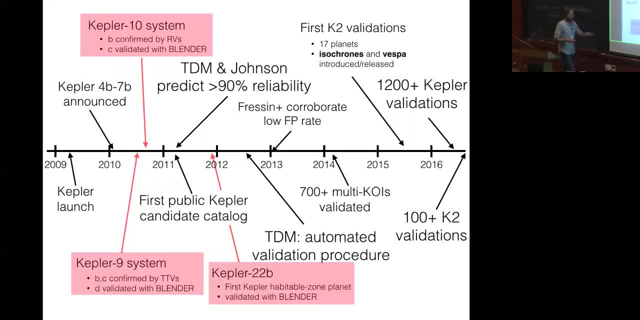 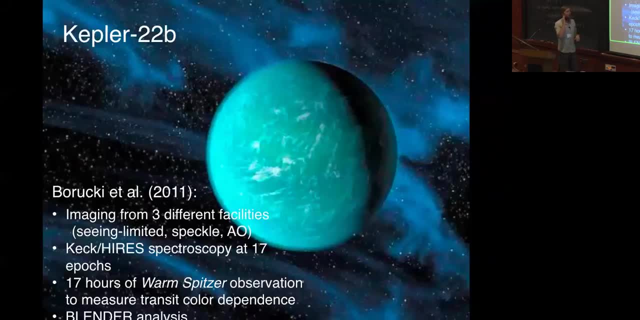 So that's what this term validation means. So again, just to give you a sense of an example of you know what went into a typical Blender analysis early on in the Kepler mission. here This is Kepler-22b. It's cut off at the bottom. 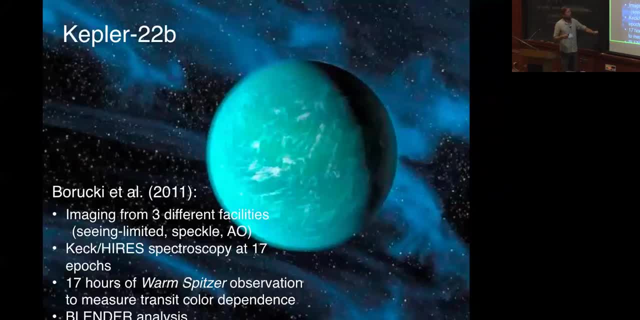 I don't know why. So the you know the end of this analysis was this probabilistic result from Blender. But what went into it was, you know, lots of high-resolution imaging, 17 epochs of, you know, high-resolution spectroscopy, the Keck telescope. 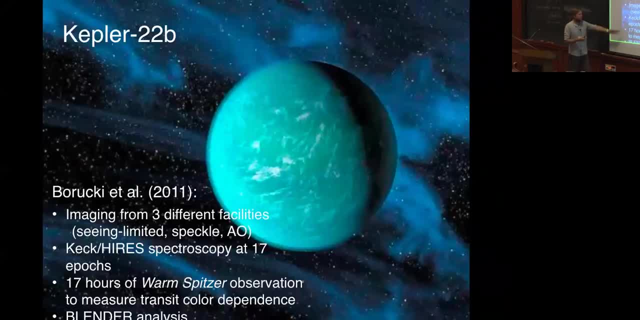 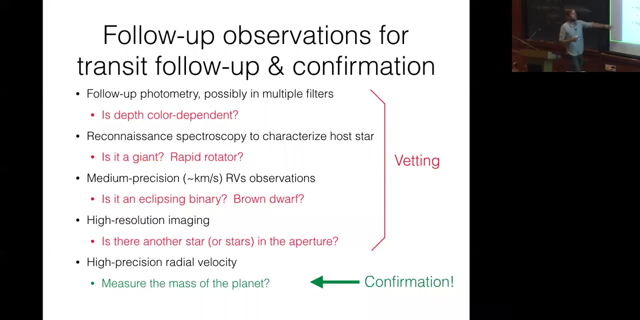 That's a lot of Keck time And then 17 hours of Spitzer time to look for color dependence in the transit depth, And then at the end of this procedure was this sort of probabilistic argument from Blender. So what Blender basically did, was it kind of left this first stage in place, where you still do all the observations that you can for a particular candidate? 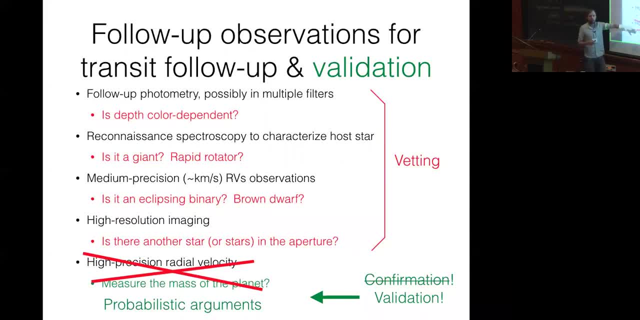 You just sort of replace the last step here. You're like: okay, we can't measure the mass with radial velocities, so let's make a probabilistic argument and consider it validated. So that's great. Except for that, we still have a problem. 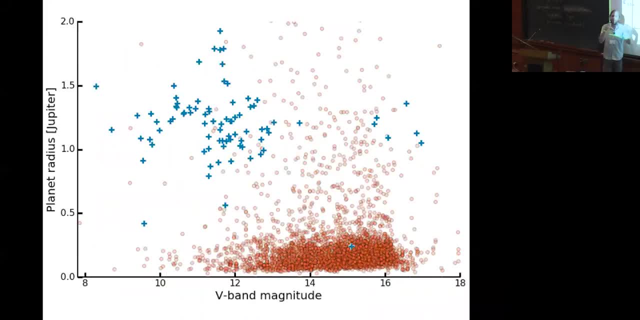 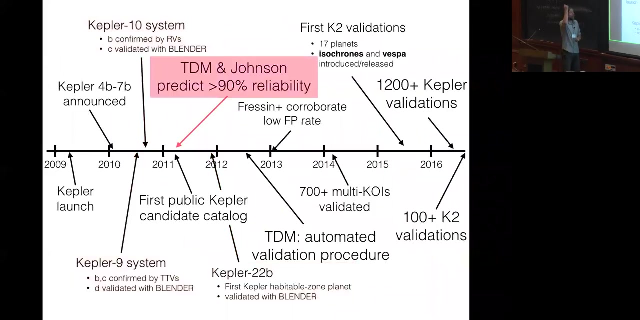 We still have thousands of candidates around faint stars And so that particular, you know, mode of dealing with Kepler candidates is not really scalable to the entire set of KOIs because the stars are faint and because there are thousands of them. So in response to that reality, so when I was a grad student here, right about the same time, 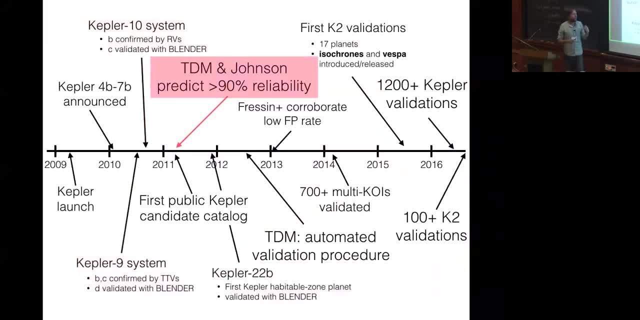 when the public Kepler candidate catalog was released, I published a paper arguing that for candidates that are well vetted. so you know I defined that specifically in the paper, meaning that the signal does not look obviously V-shaped and there's no detectable secondary eclipse. 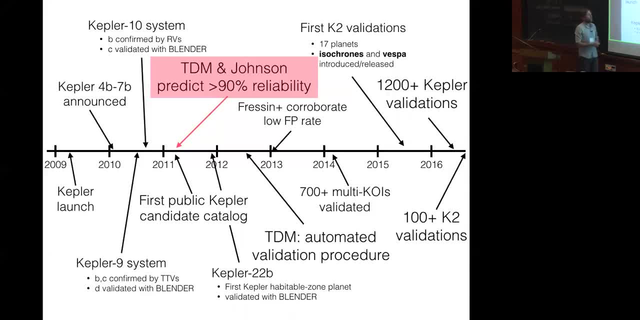 For my argument. the argument that we made was that about you know, 90% to 95% of those well-vetted Kepler candidates should turn out to be positive. So you know that was pretty exciting because you know up until this point the whole history of exoplanets. you know, transiting exoplanets was lots of follow-up observations. 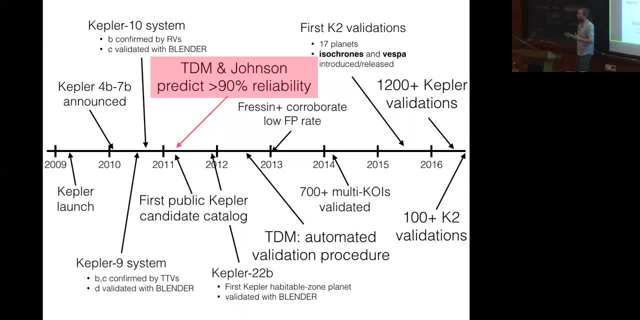 And, at the end of the day, you have, you know, the small set of candidates that you confirm is planets, But what this was saying was that most of the things that look good are probably good, And what that allowed us to do was to do statistics on the population of Kepler candidates, as if they were all planets and have some, you know. 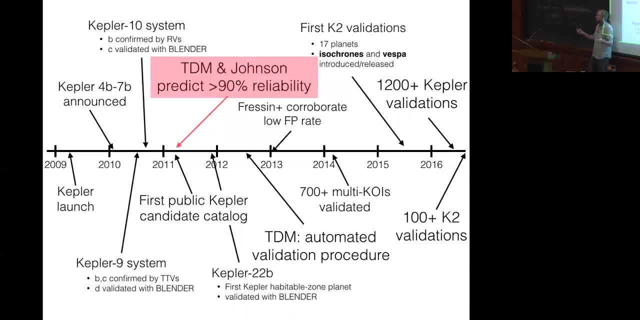 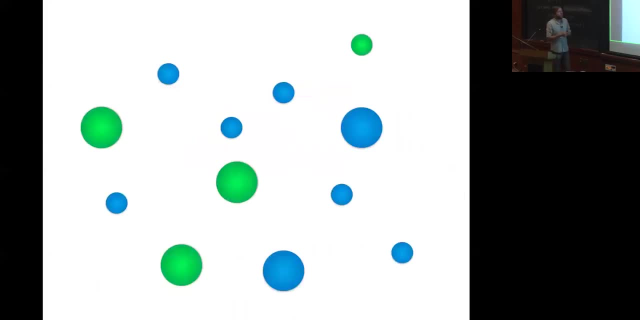 reasonable expectation that those distributions actually reflect the distribution of actual planets, even though there might be still some false positives in there, And what this analysis was based on essentially was colored marbles in a particular sense. So if you think about, you know the classic probability, you know the way you might teach probability in elementary school. 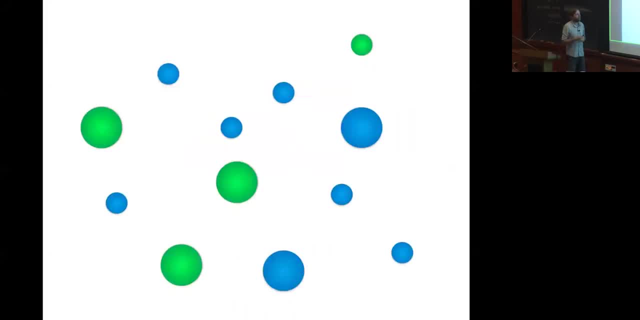 you know, is if you have a bag of colored marbles, you know, you ask like you know what is- reach your hand in and pull it out and what is the probability that this marble is going to be green? 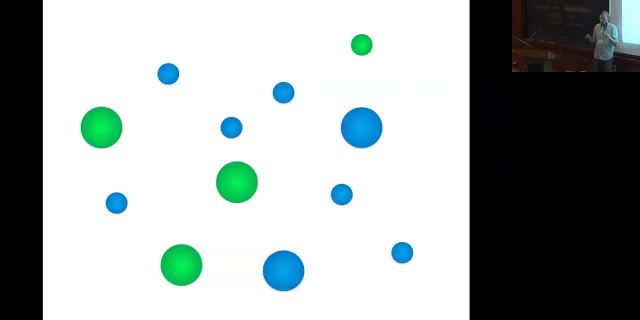 Your answer to that question, will you know. it depends on what information you have. So if all I told you is that there were two colors of marbles- there's some green, some blue- I don't tell you anything else. The best you could say was that, okay, it's a 50-50.. 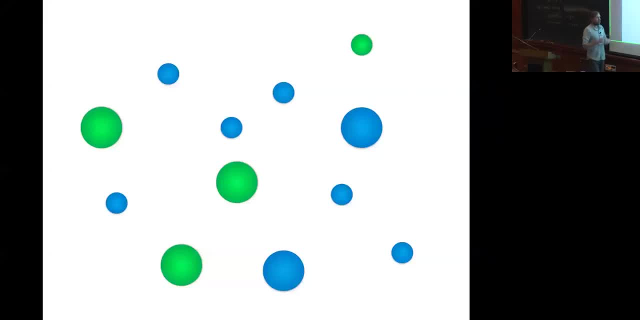 It's a shot for me to get a green marble. If I tell you more and say I have eight blue marbles and four green marbles, then you say, okay, great, It's a- you know, one in three chance that I'll pick a green marble. 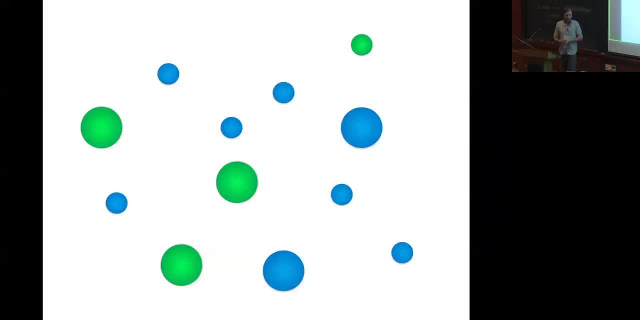 But if I give you more information and say that I can tell you that you know, three-quarters of all green marbles are large, whereas only one-quarter of blue marbles are large, then if you, you know, reach your hand into the bag and calculate the likelihood with your hand, you can tell you know. 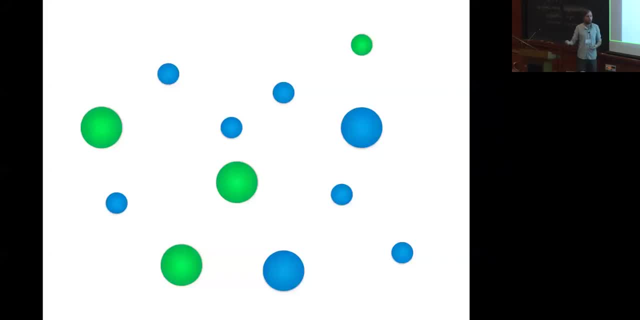 if it's a big marble or a small marble. if you feel that it's a big marble, then you know that there's a three-in-five chance that it's actually green, even though only one-quarter of the marbles in the bag are green. 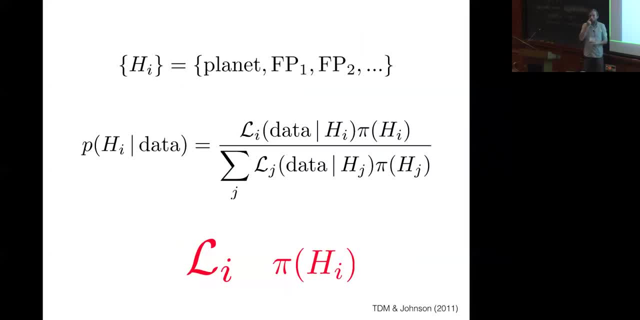 So this is exactly analogous to what we did with exoplanets and false positives- astrophysical false positives. So this is this should look familiar from Tom's talk this morning. This is Bayes' equation here, Where we're talking about the probability of a specific hypothesis conditioned on the observed data. 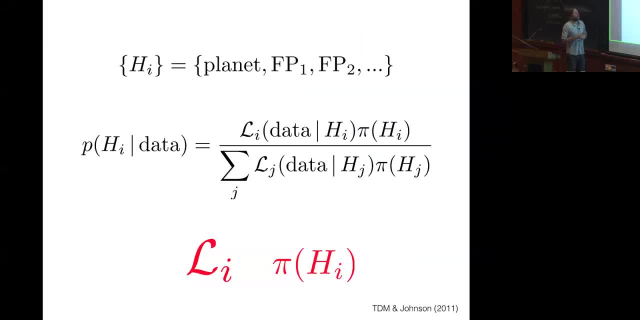 And the hypotheses we're considering are that your candidate is caused by either a transiting planet or one of any of a number of specified false positive models, And the way that you calculate the probability that, the probability of the planet model being the true model, given that data, is this: 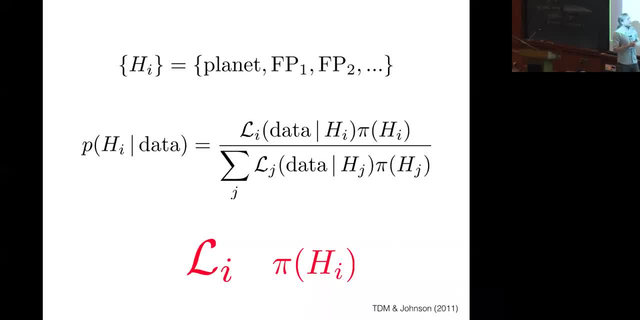 You have a model likelihood, a model prior, and you divide it by this marginalized likelihood over all of your models. So this is the likelihood of each in each model, under each model, weighted by the prior of that model occurring. So what we do here is just, you know, come up with astrophysically motivated priors for all these populations and calculate the likelihoods. 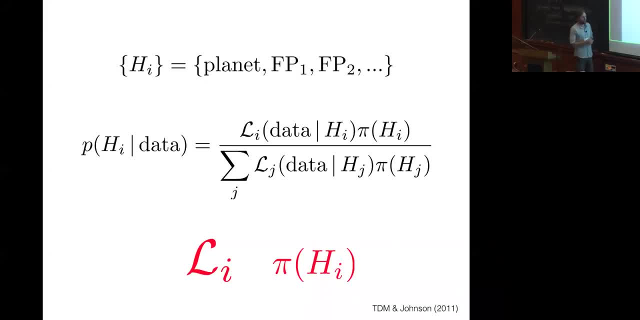 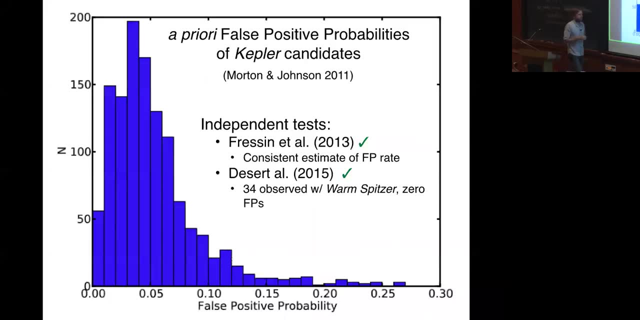 you know, in some sensible way, which I'll talk a little bit more about in just a minute. So so the end result of this was was that, you know, we predicted, you know, the false positive probabilities of Kepler candidates would be generally low. 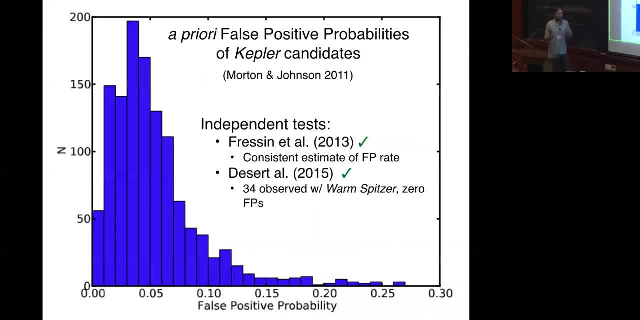 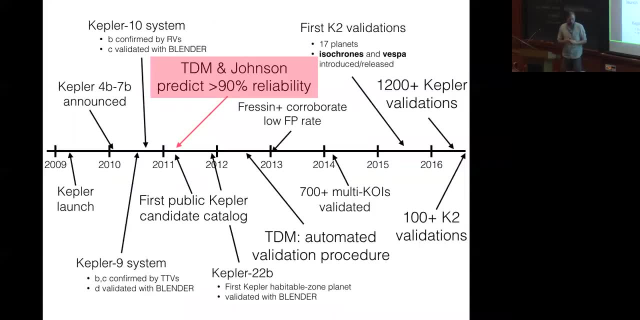 And this was subsequently verified independently, both theoretically and observationally, by by these various studies. So sort of like moving on past the sort of initial exploration that we did in 2012,, I came up with this a little bit more sophisticated procedure. 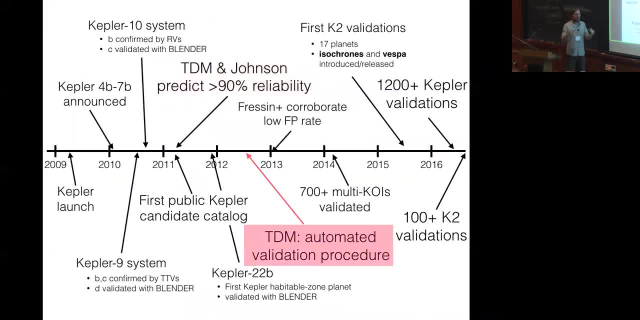 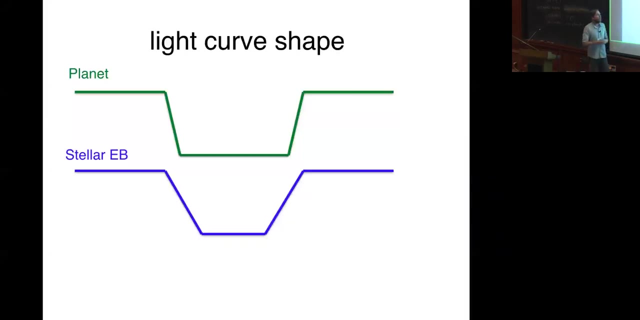 To take into account a little bit more information about the, the, the, the light curve in calculating the likelihood, for you know, under the the, you know what I just described, under the Bayesian formulation there, And what this is based on was again this kind of intuitive sense that we all have, that you know, planet transits are typically boxy. 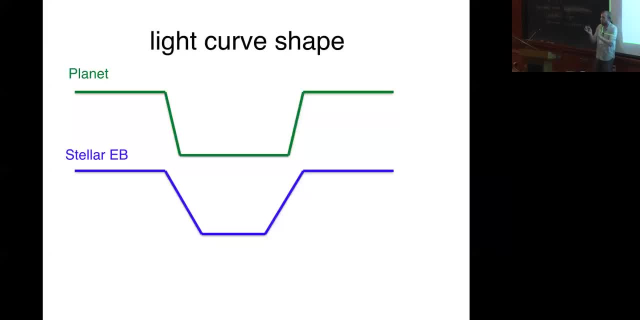 And if you have an example of this, you know, if you have an example of this, it's an eclipsing binary, it's more V-shaped. So you know you can how Rafael was showing those Kepler candidates earlier And you know we all sort of had the intuition that the ones that are kind of rootshaped looking, those are probably false positives. 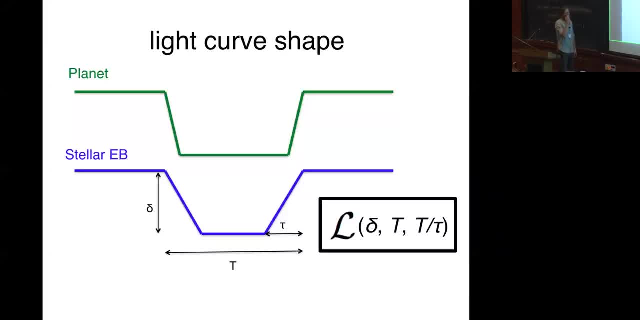 What? what this allows, it allows you to do, is just sort of put numbers to that intuition. So I defined a. you know this particular sort of artificial model for a transit, which is a trapezoid shape And it's kind of like a На. 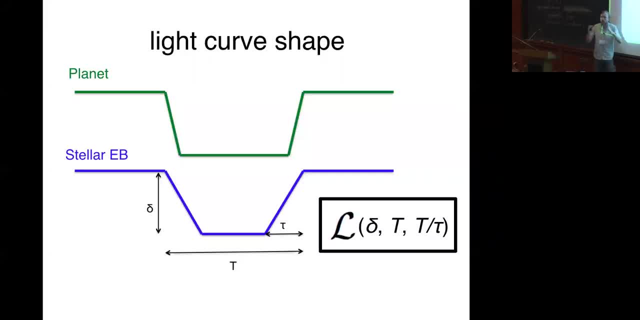 It's like a Neon sort of minimum kind of parameterization that characterizes the most important features. So you have a period, obviously, and then the depth of duration and the kind of v-shapedness parameter. And what I did was simulating representative populations of all these scenarios and sort of measuring what is the typical. 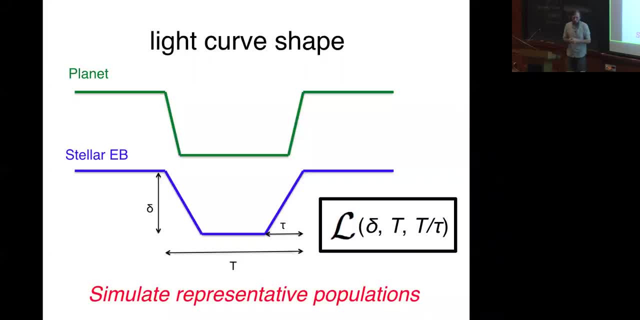 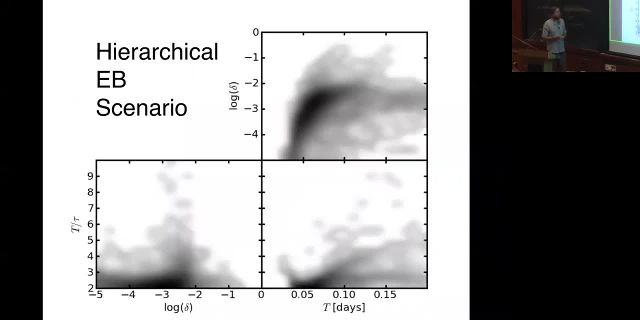 distribution of these shape parameters under the different scenarios And that's what we used to calculate the likelihoods under the model. So you know just very roughly, this is you know kind of what things look like. These are three different projections of this trapezoidal parameter space under this. 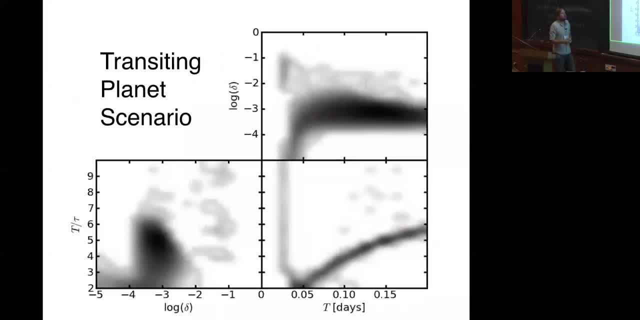 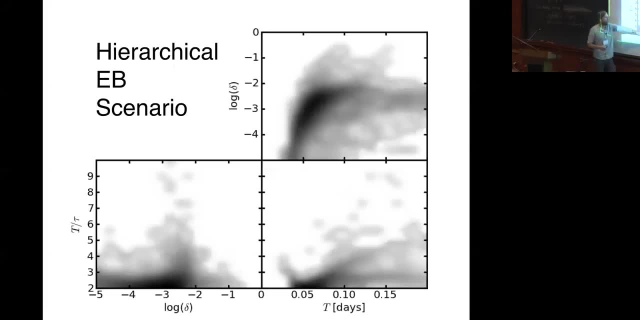 is under a hierarchical eclipsing binary scenario and this is for a planet scenario. So you see that this sort of occupied different regions of this parameter space, especially, you see that the eclipsing binary stars tend to be more v-shaped. This is t over tau equal to zero. 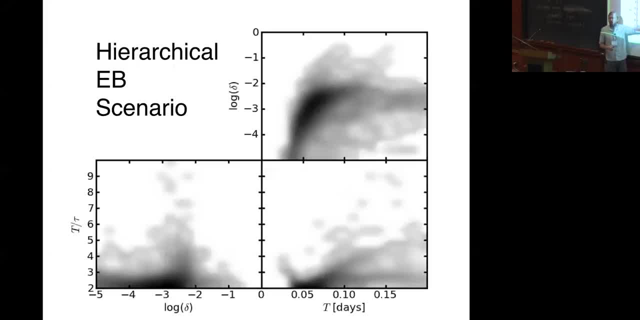 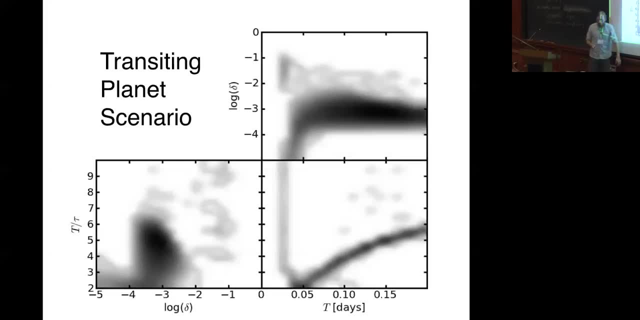 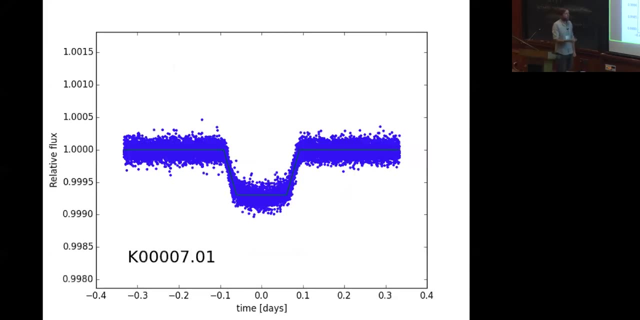 Two is the, the v-shaped line, and so the eclipsing binaries tend to be much more v-shaped and the planets are more boxy, which is up here For a specific example? this is KY7.. I think this was. this is one of the first Kepler detections. 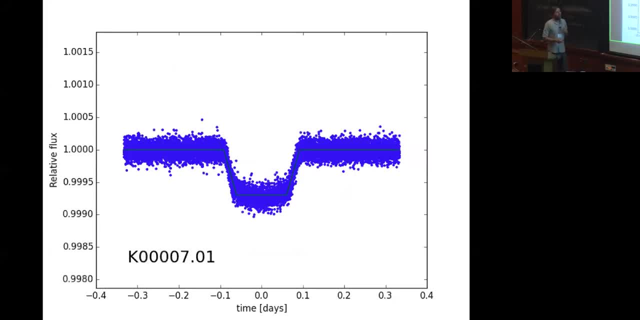 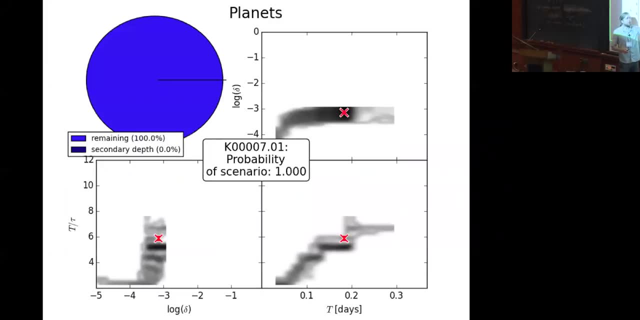 It's nice boxy, nice boxy looking signal. It lands right here. The X is the measured trapezoidal shape parameters of the actual signal, and then the fuzz below is the, the model simulations. and it doesn't do well in all the other false positive scenarios. and when you put all this 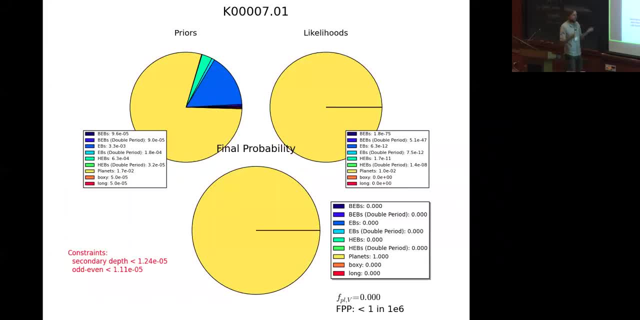 together. you know that you end up with a final probability that this thing is caused by any of these defined false positive scenarios of like less than one in a million and the the. the thing about this in particular is that you know this statement is made without any follow-up. 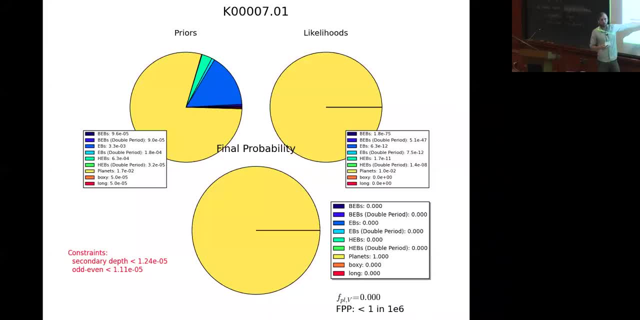 observations at all. This is just based on the data from the Kepler space telescope. so there were, you know, the. the vetting procedure that turned the original detection Kepler into a planet candidate by Kepler was looking for things like the centroid offsets and the secondary eclipses and all that that's. 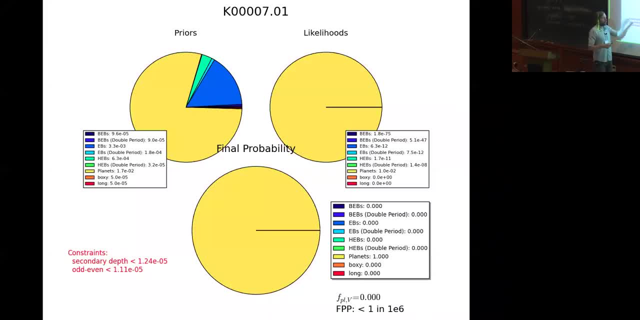 that's all taken care of, and then we have the shape of the photometry and just based on the shape we can say it's less than one in a million chances to be a false positive. So this we can call a planet without having to do any follow-up observations. 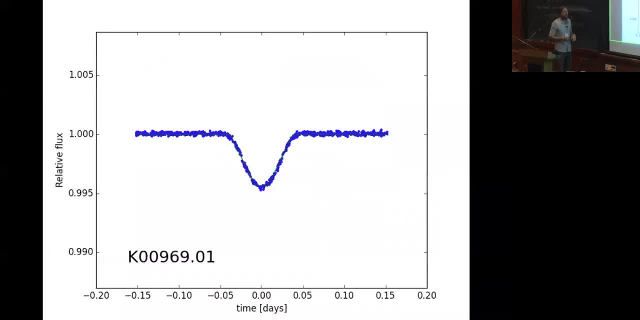 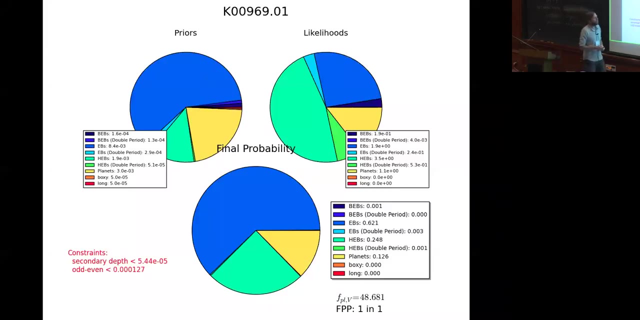 I'm glad that's the innovation of this, and this is an example of something that did turn out to be a false positive observationally, and you can see it looks v-shaped, but when you put numbers to this, you know you get something like a. you know two and seventy five percent, eighty percent chances this is going to. 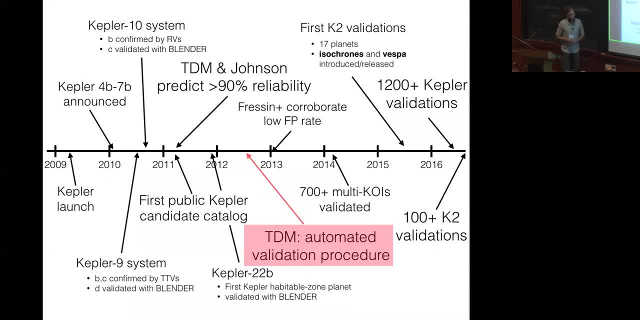 be a false positive, and it is so. that was the. so this, this automated validation procedure that I wrote about originally in 2012, eventually put it into a couple of software packages called isochrons and Vespa. Vespa is the tool actually, both of these tools you'll be introduced to in. 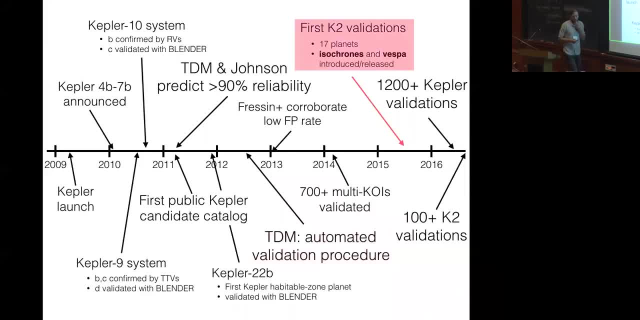 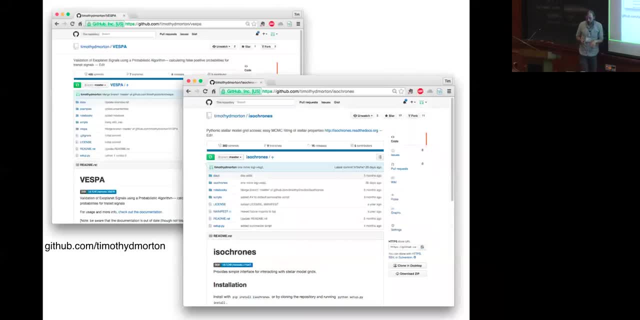 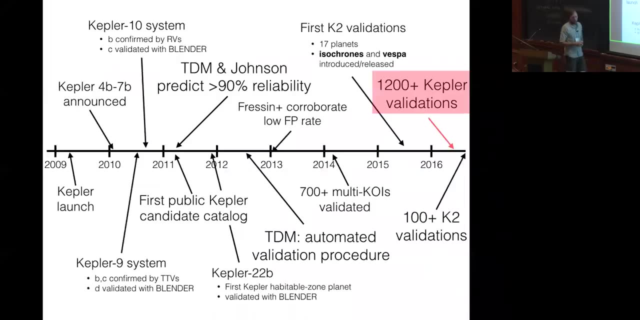 the hands-on sessions starting tomorrow. they're both publicly available Python packages. you can just install them. you can get them from github and I applied the Vespa code to all of the Kepler candidate and that enabled us to turn. this is the population of all the Kepler candidates. 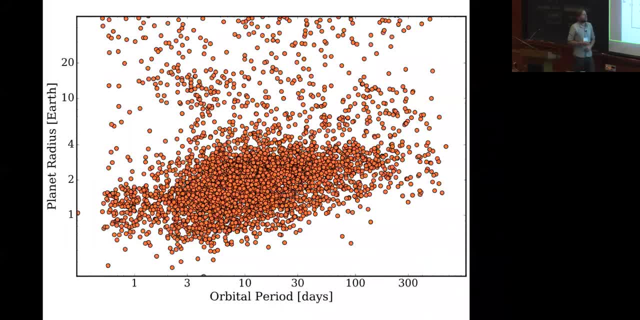 from the you know the that existed in, like the second-to-last data released from Kepler planet radius versus orbital period, and when you sort of fade things out by their false positive probability, you see that things that are likely false positives disappear and you get, you know, you're left with just the. 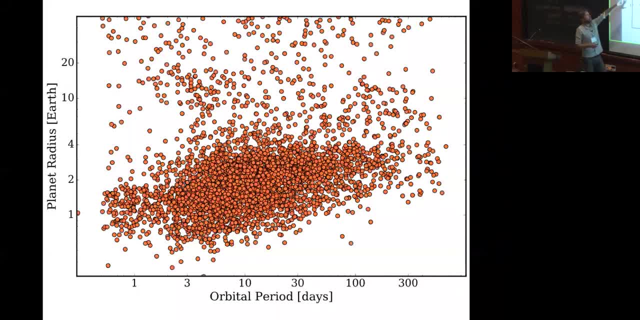 things that are likely planets, which is, I think, in particularly, what I'm going to talk a little bit about right now is a kind of a rule of thumb. So you can see right here, it's a bunch of false positives that disappear in the region of the Kepler planet. so it's. 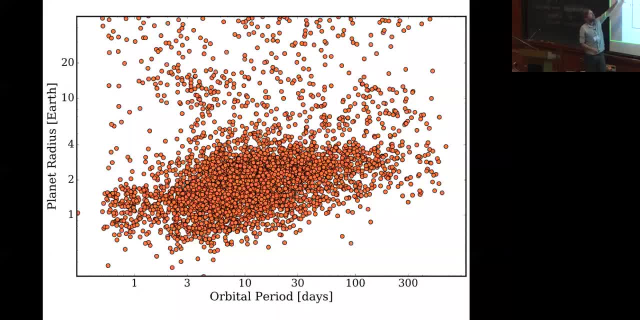 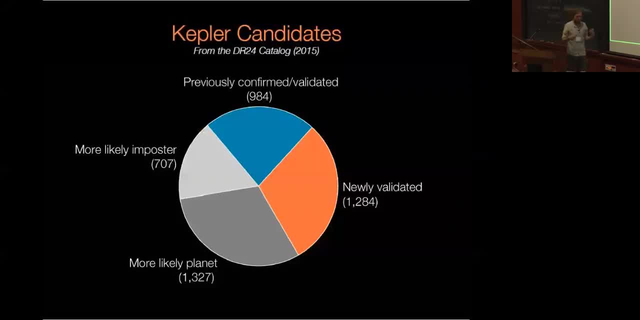 something called a super mercury. this is a really interesting thing to see, is, what's interesting is this sort of evaporation Valley right here, like false positives disappear from that and then there's like this, I think is like evaporating super mercury. so it's like one of these weird, weird things up there. 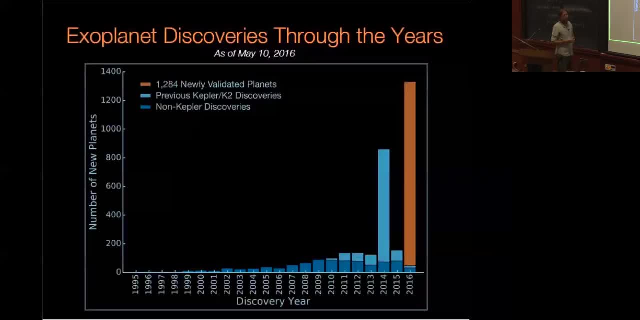 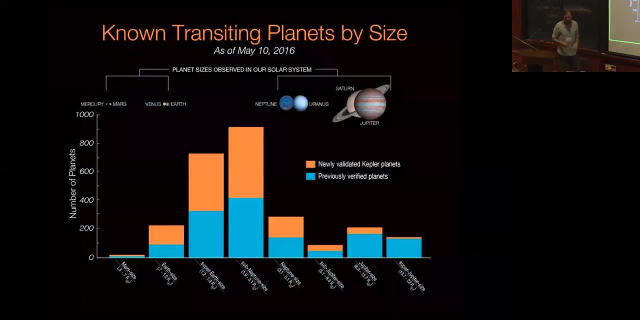 but you know, the false positives disappear from that region, which is kinda cool. 1,200 planets, This is a fun figure to make you know. yeah, anyway, And this is the additional, you know we've more than doubled the number of known planets. 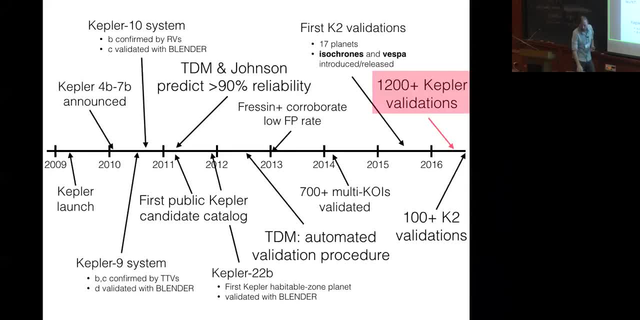 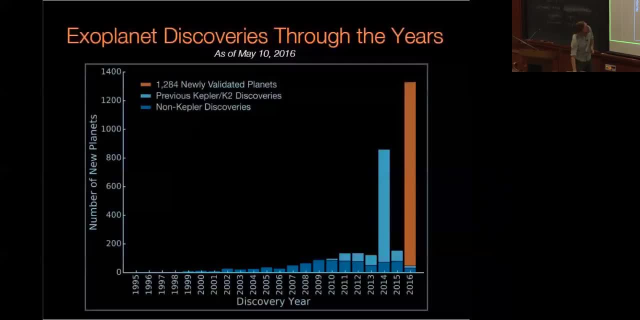 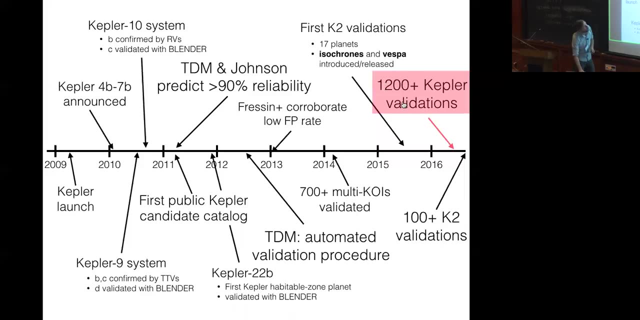 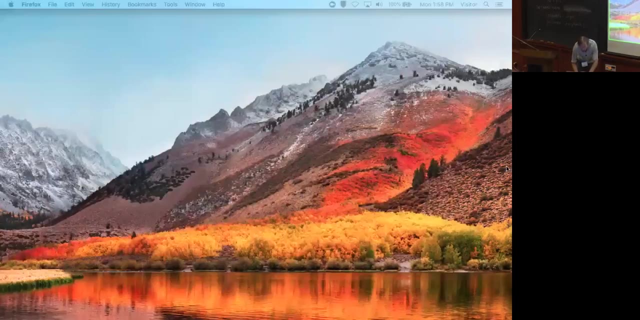 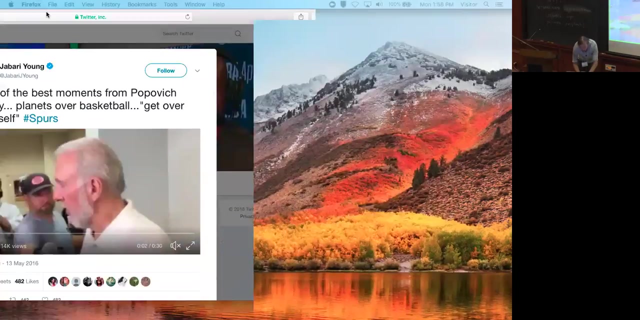 smaller than Neptune. And then I'll end mostly with: there's a link. yeah, okay, So this was from. so this announcement was made. sorry, it's on my screen. one second, one second. hold on, Let me drag this over. This was made. 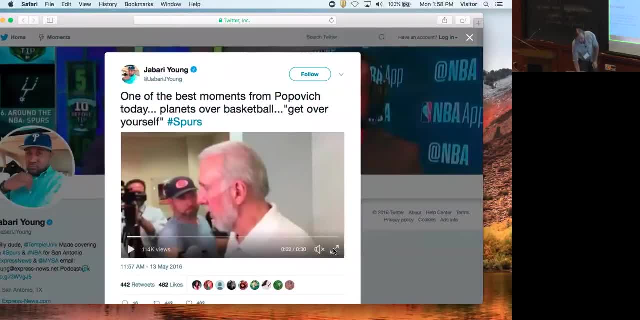 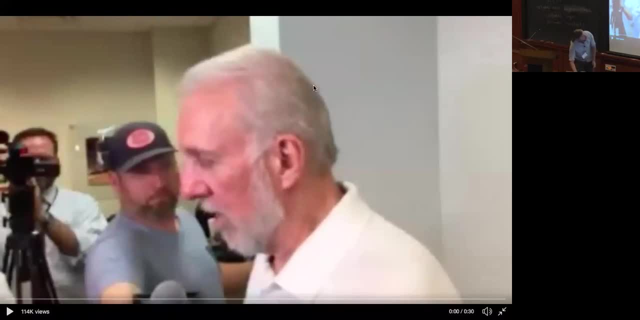 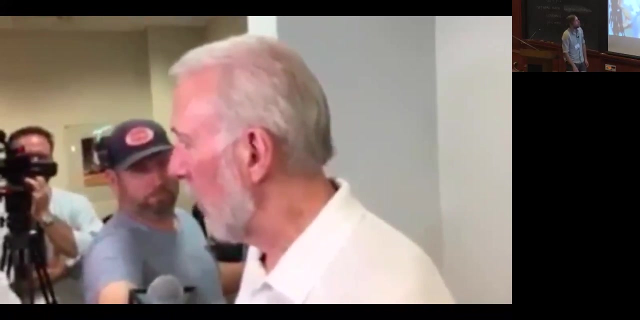 during the NBA playoffs in 2016,, and so you may recognize this as the head coach of the San Antonio Spurs. This was in a post-game interview after the Spurs lost the game, And I'll play this. I'll try. NASA discovered all those habitable planets the other day. do you guys know about that? 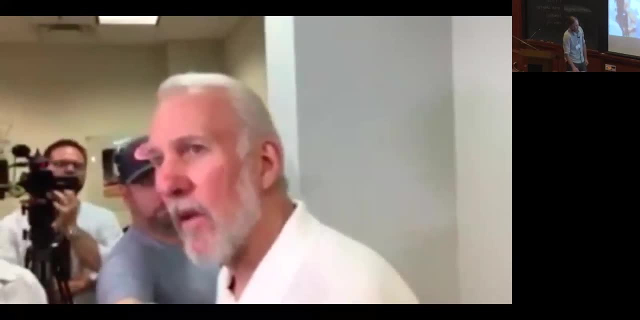 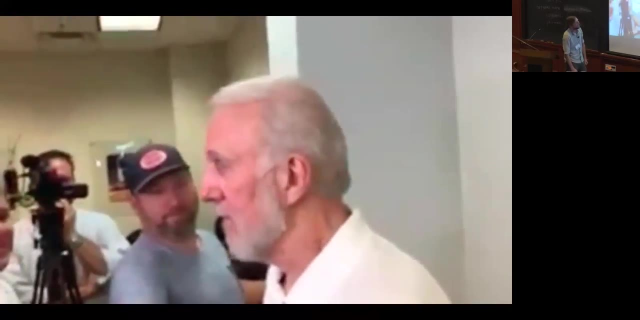 Yeah, What did they say there were how many of them? 1,200, I think. 1,200 habitable planets- Well, 1,200 in New York. And then last night somebody lost a basketball game. That's not true. 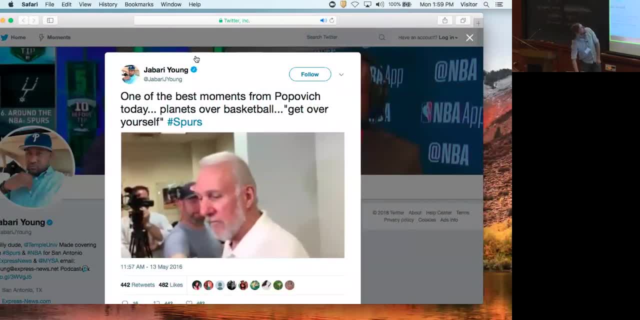 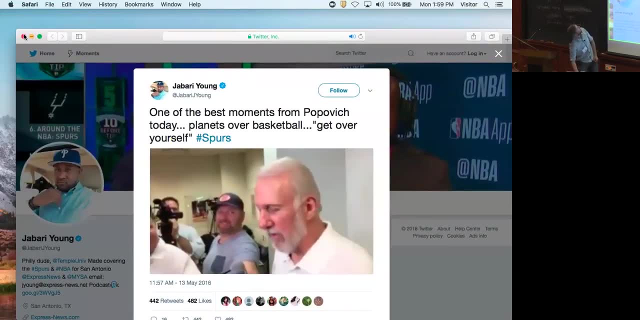 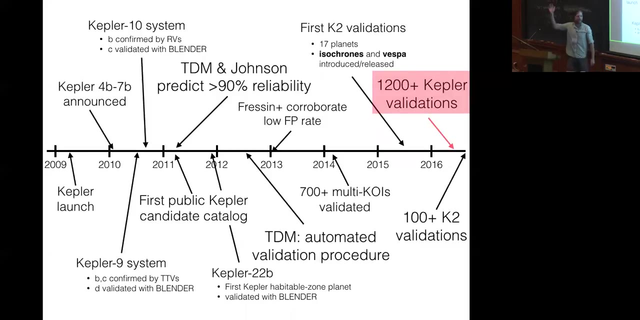 I don't want to answer your question. You're a radio talk show guy that just stirs it up, Anyway. so that was my, like you know, two seconds of the same. That's my NBA career right there, But that's. that's basically all that I have here. 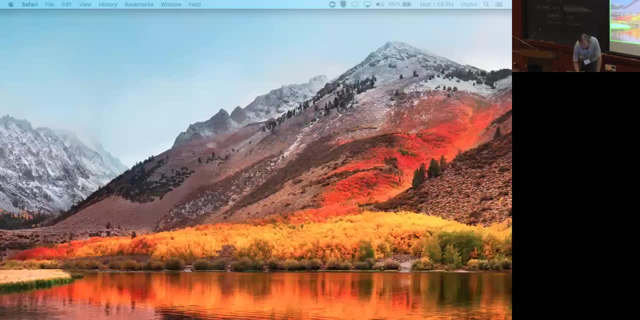 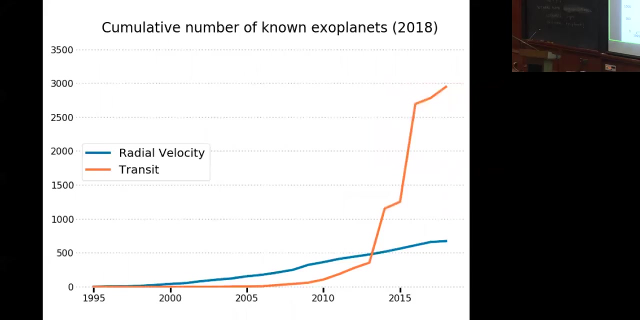 We went from wait there was I had there's one more slide actually, Sorry, Right, so again, you know, in order to get from here to there, you know, in here was a sort of complete shift in sort of how we, what we allow to be called a planet. 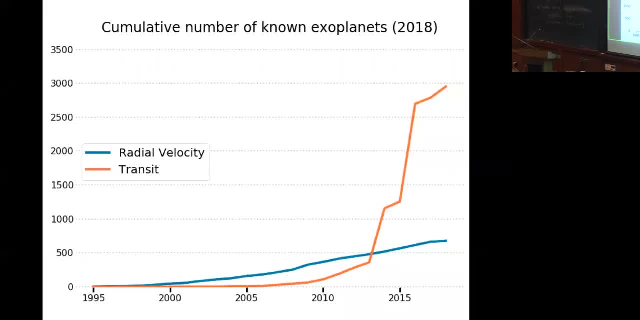 You know where. you know we started at the beginning of Kepler. we started getting comfortable with the idea of probabilistic validation And then, you know, the tools that I developed enabled this to be applied to all the Kepler candidates. And that was the big hockey stick there. 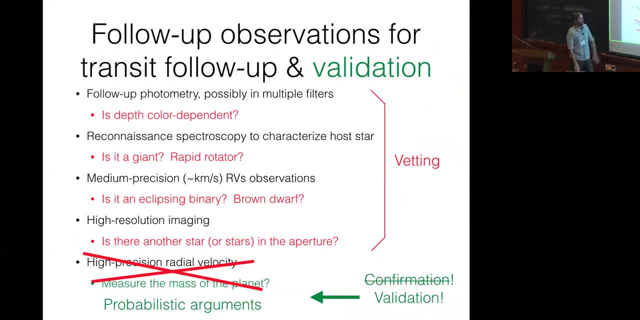 So what? what happened here was like, you know, this is what we looked, what it looked like with Blender And basically you know, we cut out all of that annoying telescope stuff to say that we can actually go straight to calling something a planet without even having done any follow-up observations. 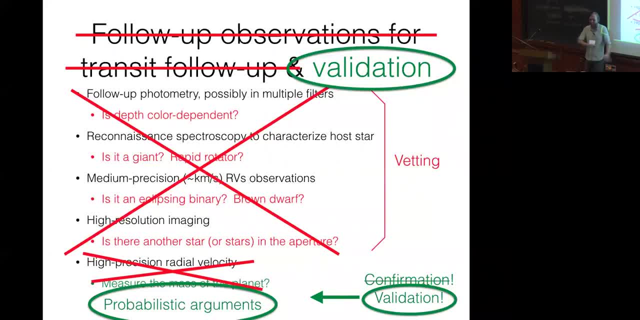 Now not to like say that there's no use for random velocities. No, there's obviously a lot of science that you know can't be done if you don't have the follow-up observations. You know you can't get planet densities without masses. 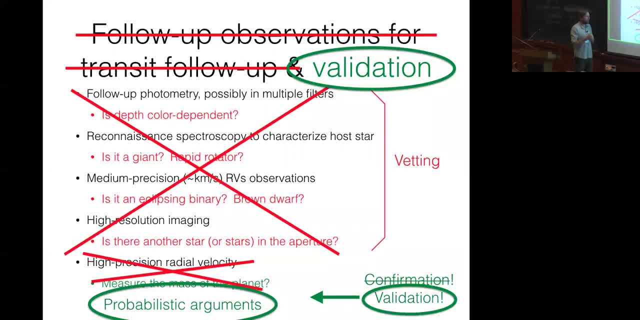 You know, and obviously if you want to learn about atmospheres you have to do careful observations. But if, if the, if your main interest is looking at the sort of population distributions of properties that are derivable from transits alone, then you know, probabilistic validation is very useful in sort of getting you there. 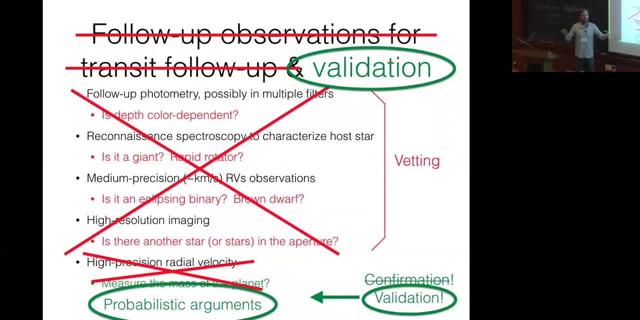 And this is sort of where we are in the field And so that sort of helps hopefully helps understand how we get there, And so that sort of helps hopefully helps understand how we get there And so that sort of helps hopefully helps understand how we get there. 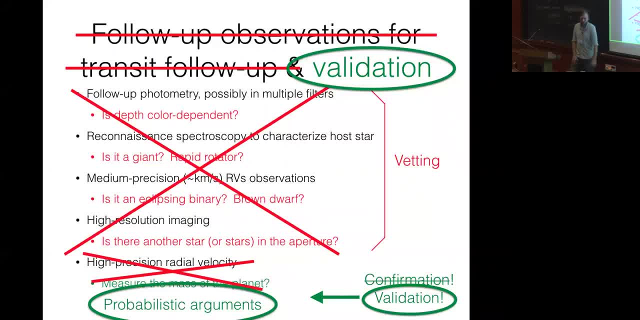 That's all, Thank you. Thank you, We have about five minutes for questions. Any questions for Tim, However, they are Right, so okay. so the question was just to clarify what the difference between confirmation. 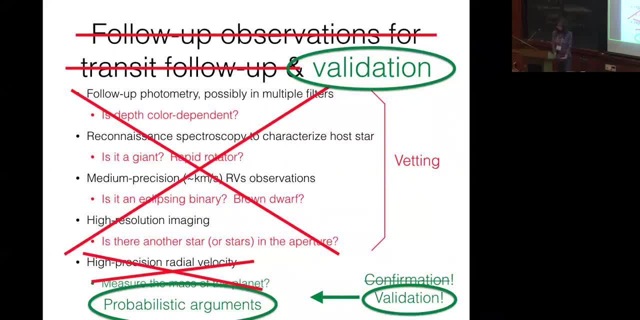 and validation is one more time. Confirmation is: you know beyond a shadow of a doubt that there's a planet because you measured its mass, either rate of velocities, transit time and variations. Confirmation is: you can also know beyond a shadow of a doubt. you know, but it's based. 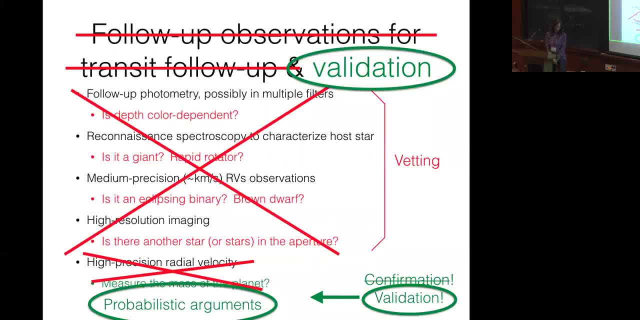 on. you know your Bayes equation has priors in it and you only define a, you know, limited set of models. So you know, a good example is that you could have a planet that gets probabilistically validated using VESPA. that is actually a instrumental artifact because you don't have. you know. 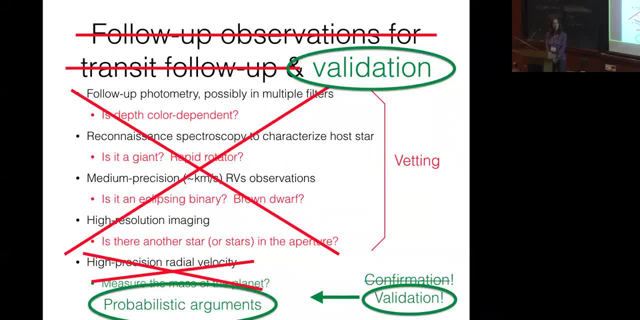 I'm not modeling instrumental artifacts as one of my hypotheses And so, like you know, like Bayesian analysis is great to like sort of select between different models, but the, you know, limitation of that is you have to in order to have like pure. 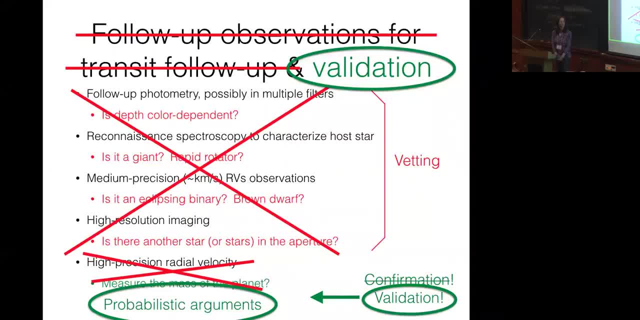 belief that you are completely right. you have to believe that you have enumerated all of the possible models. So you know, if it's something that you didn't model, then it might be there. So there's always this sort of those kind of questions and actually speaking to that, 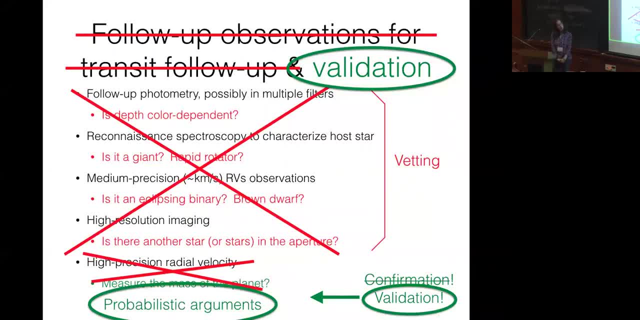 there have been instances where planets were probabilistically validated And then they turned out not to be planets, And if you come to the VESPA sessions, we'll talk more about those in the group project. Those were actually not based on just probability. 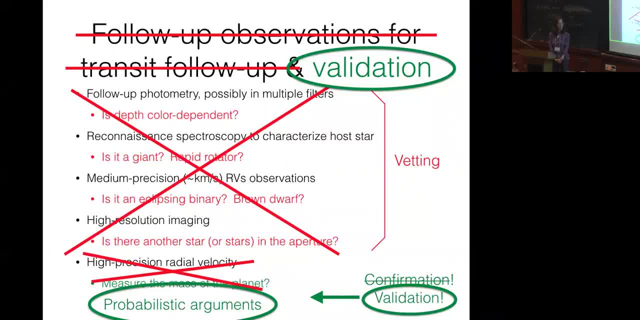 That was actually sort of incorrect application of VESPA. But you know that's more detail than we can get into right now. Any more questions This side Here. Yeah, It's a Okay, Yeah, Yeah. 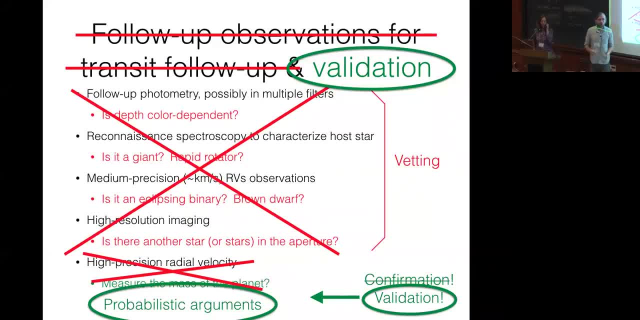 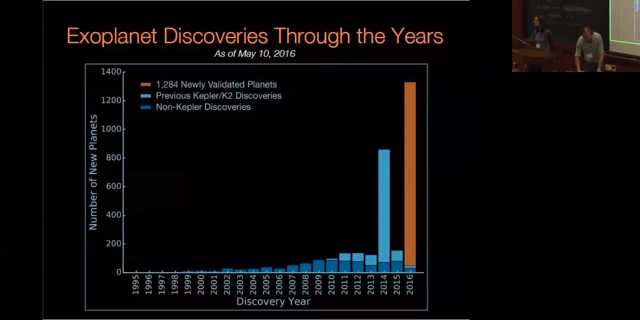 Yeah, Yeah, Yeah, Yeah. So the question was about BLENDER. Is BLENDER an acronym? Is it a method? It's the name. I don't think it stands for anything. Is there a way to? Let's see? 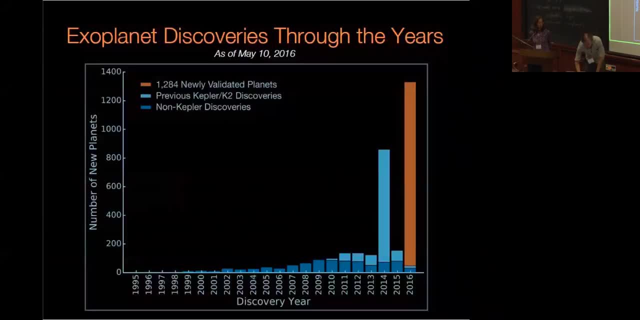 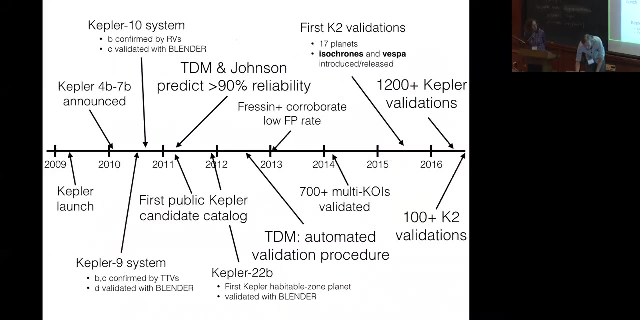 So I skipped the slide with details of BLENDER. But if you were around exoplanets circa BLENDER era, did it disappear? Does it show hidden slides? Do we know how to show hidden slides here? Anyway, I had a hidden slide. 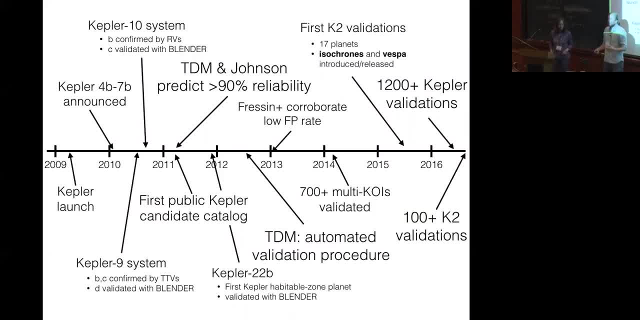 I have a hidden slide on BLENDER But I can talk about it. It's another. It's a procedure that fits It like looks It tries to like simulate every possible false positive And like it doesn't simulate false positives. 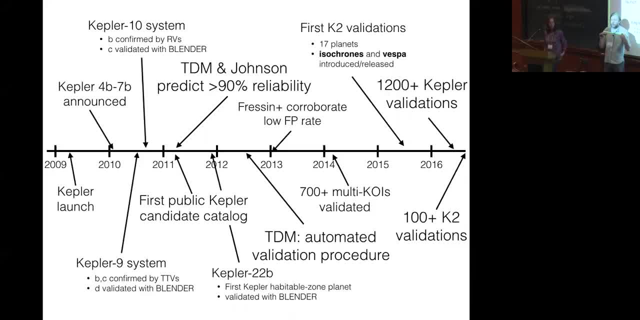 It defines a false positive model, It gives you the best fit of the data according to that model and sees, you know like what region, In what region of false positive parameter space do the false positive models give you? you know, as good a fit as the PLANET model, roughly defined. 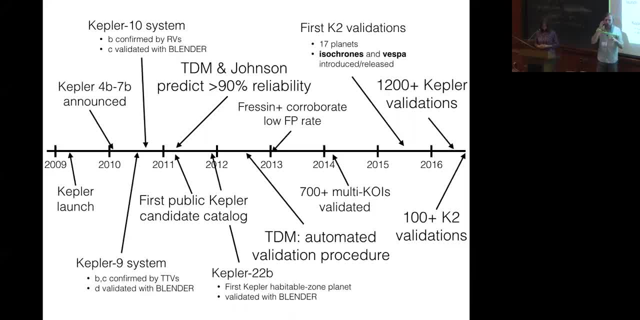 And then after doing that, then you look at. you know, can I chop away at that parameter space by the follow-up observations that we're doing? So that's So. it's similar in spirit to VESPA, but VESPA is a little bit more rigorously sort of defined.